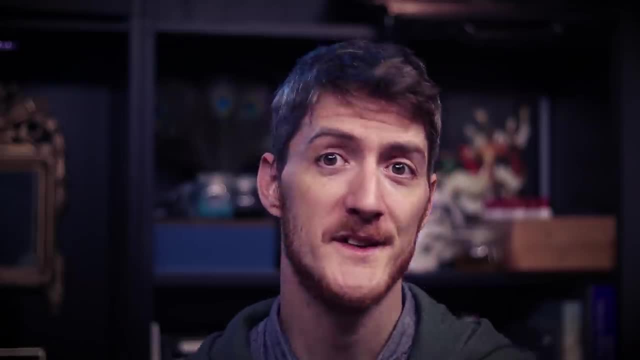 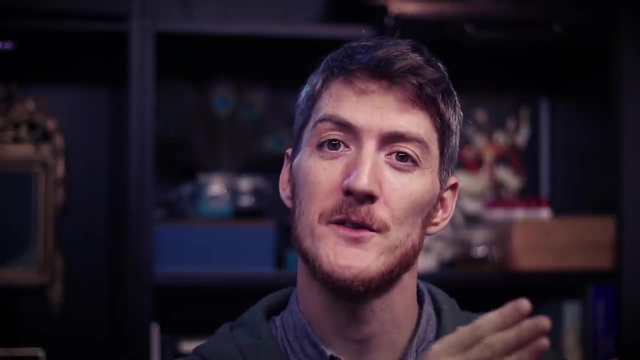 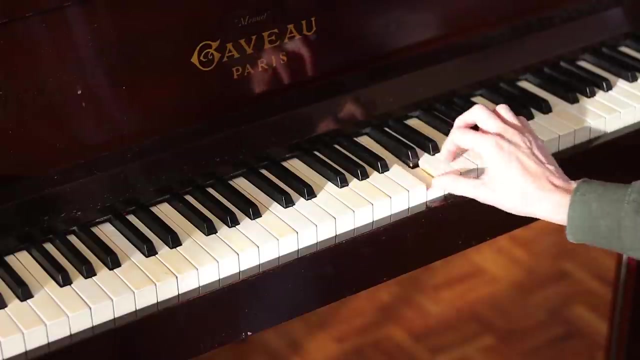 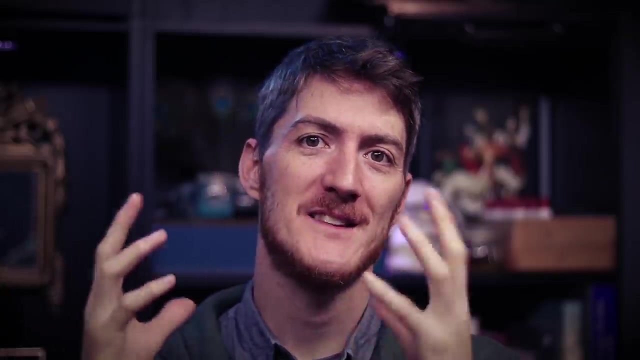 other. It's a little bit like music: if you just have one sound, it doesn't make a note. but if you have an organized system of sounds, it creates music theory and all of a sudden the sound actually become notes. Without a coherent classification system, we just have visual impressions, and color is more. 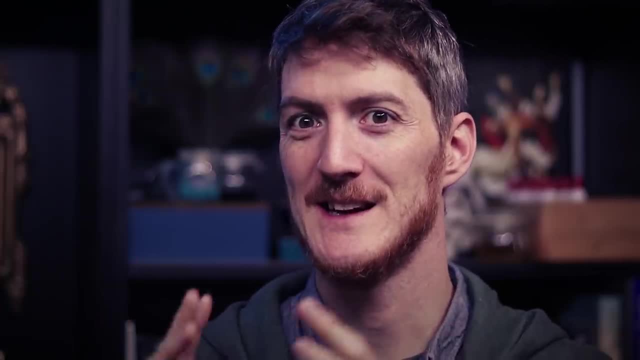 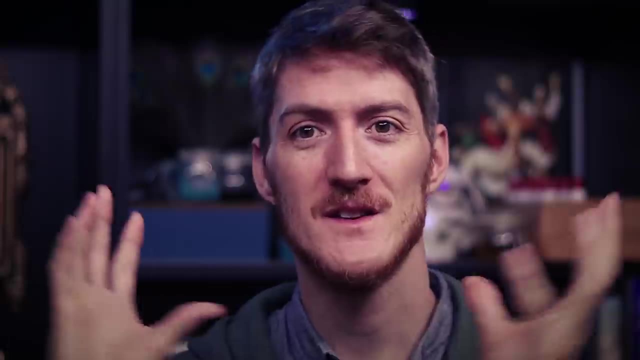 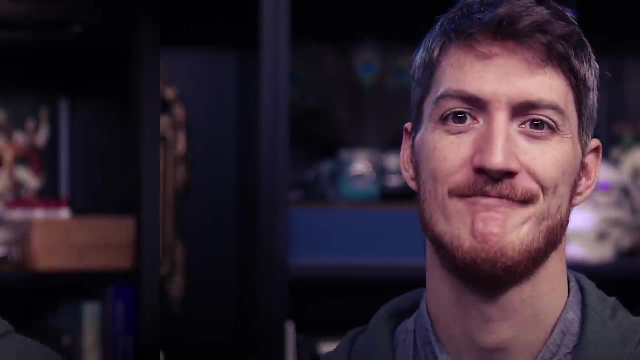 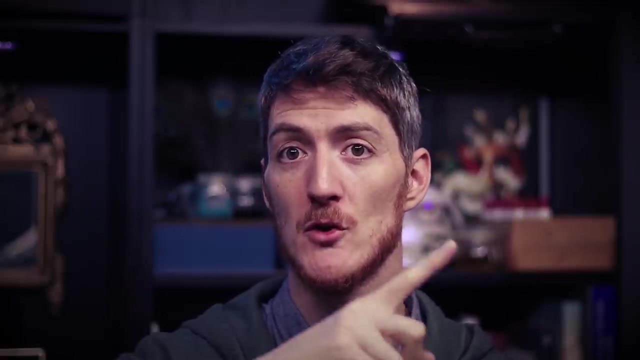 of a guessing game. Artists, painters especially, need a lot more accuracy, and in this video I'm going to present to you a system that considers color in all its dimensions, dimensions that are often forgotten. The second role of color theory is to explain how to mix and transform colors, So how to go from one color to the other. 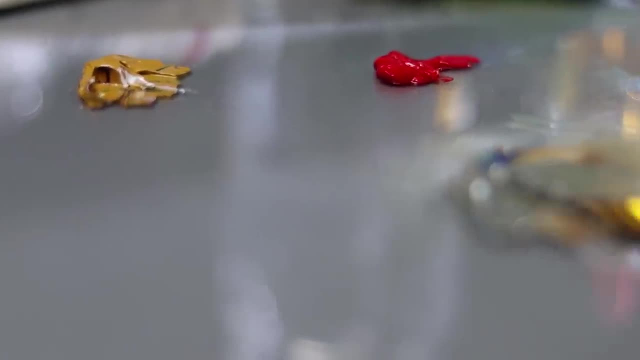 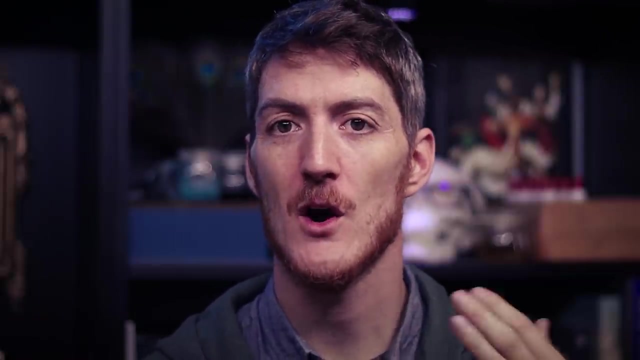 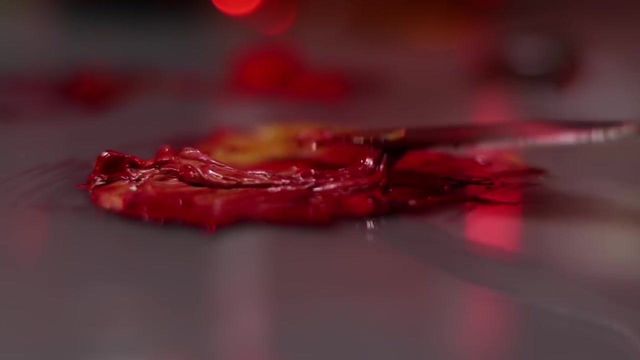 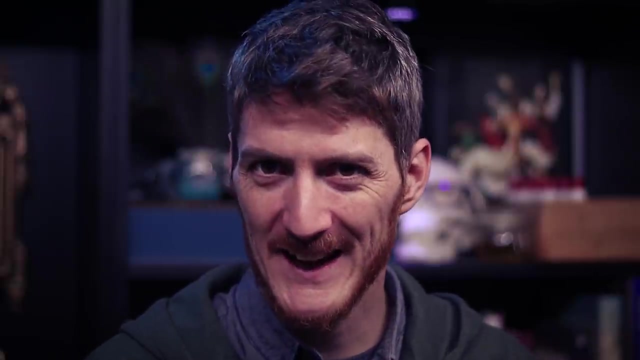 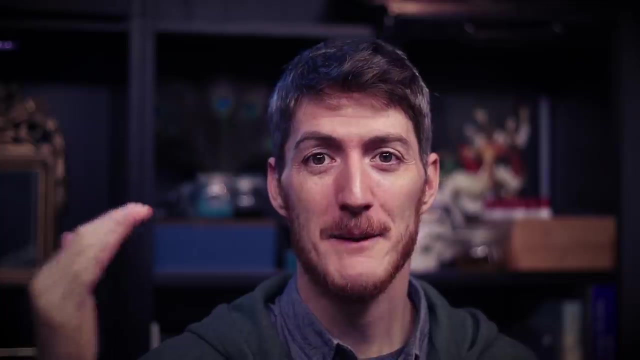 When we are painting as artists, color is not a static thing, it's a dynamic thing, It's constantly evolving and color is constantly transforming itself. And it's really easy to lose track. because, Because being a painter is a little bit like being a musician, who would need to tune the instrument while playing and invent and create the notes as they go into the song. 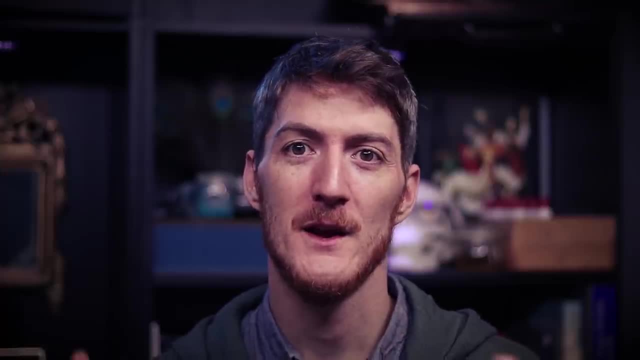 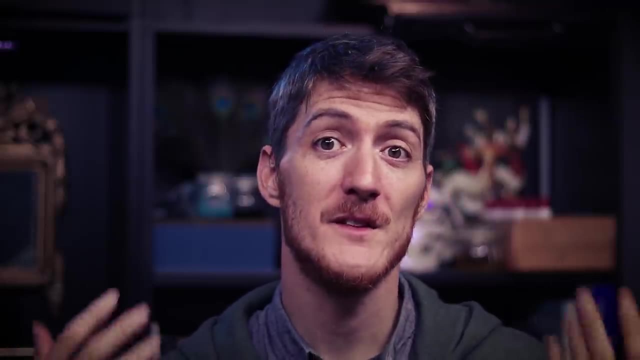 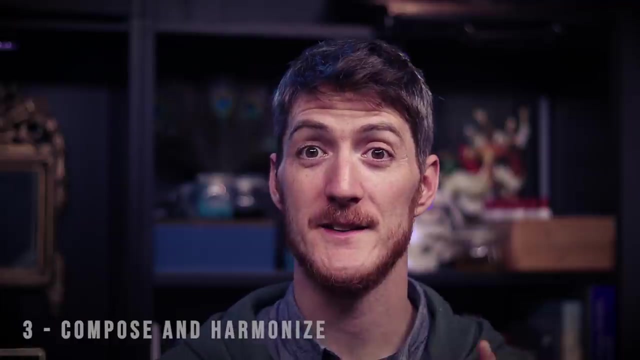 And painters need a very structured and methodical method to approach this constantly evolving existence of color, And this is why color theory has an important role to play there too. And the third major role of color theory is to explain how to compose and harmonize colors. 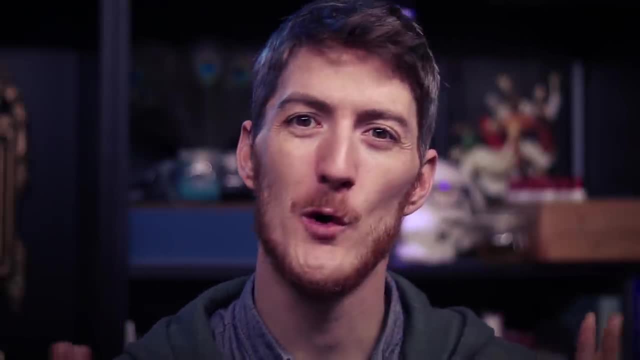 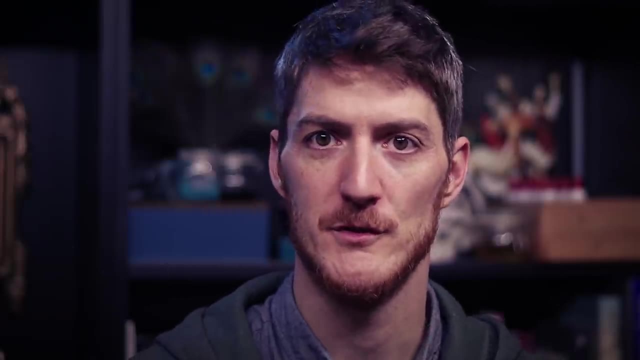 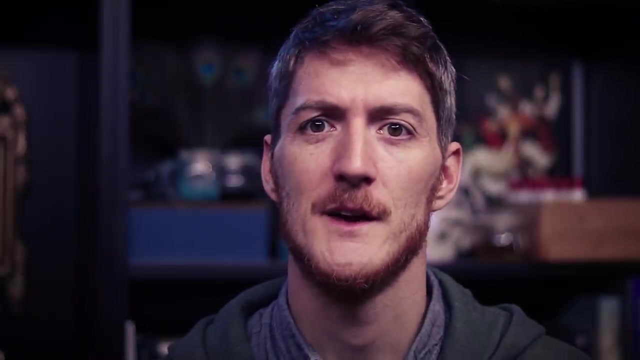 Unfortunately, this part is widely overlooked nowadays. Most of the time you would hear: well, it doesn't matter really, which color you place next to another. Well, it's all subjective. You hear a lot of things like it's all relative, anything goes. 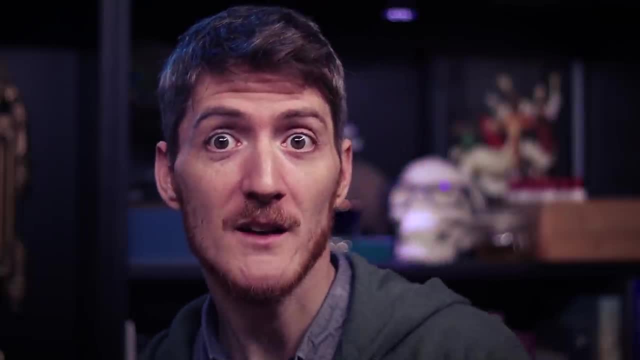 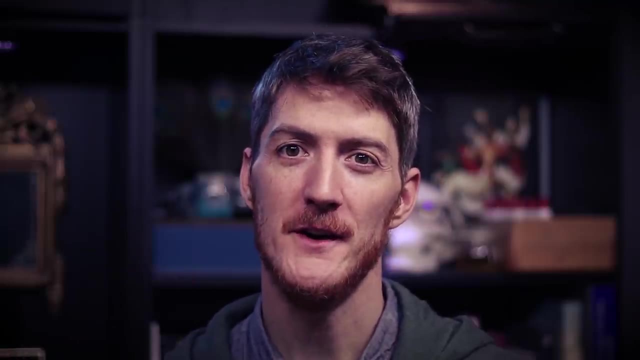 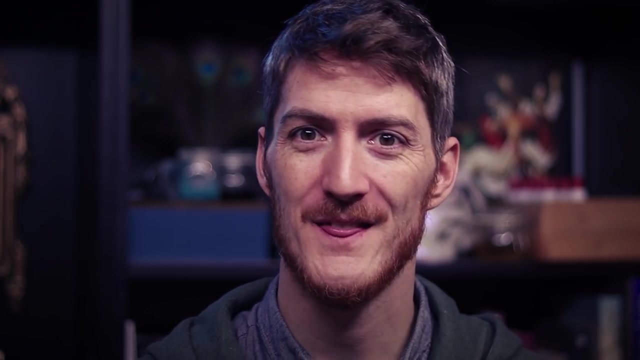 And yeah, it's true. in a way Anything goes. And it's weird because here music still has a very well-defined harmonic structure. In music you don't put any two notes next to each other. Some notes go better together and they form chords. 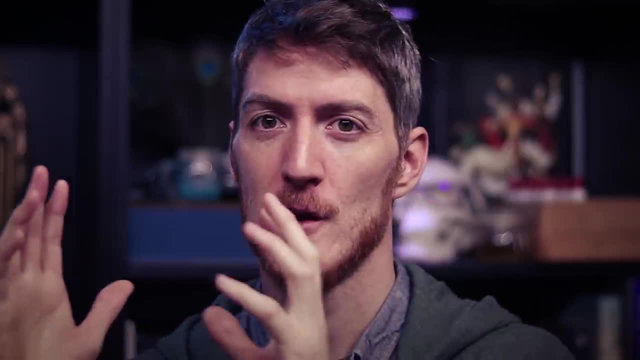 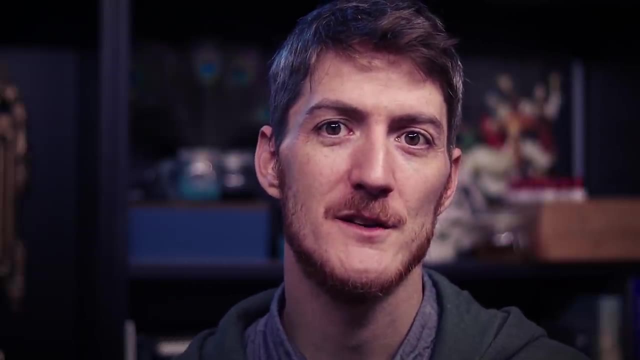 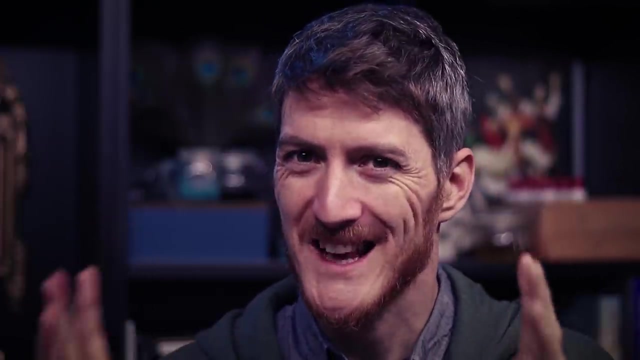 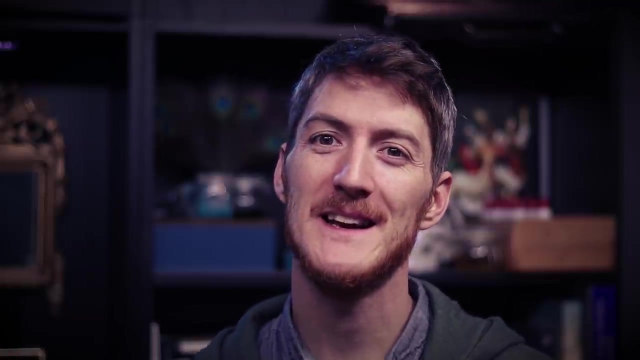 And with a very limited set of chords and notes, actually you can create limitless numbers of combinations for musical compositions. You can go from classical to heavy metal with the same set of chords, And I think that really it's a shame that the world of visual arts have completely given up on the idea that there could be chords for colors. 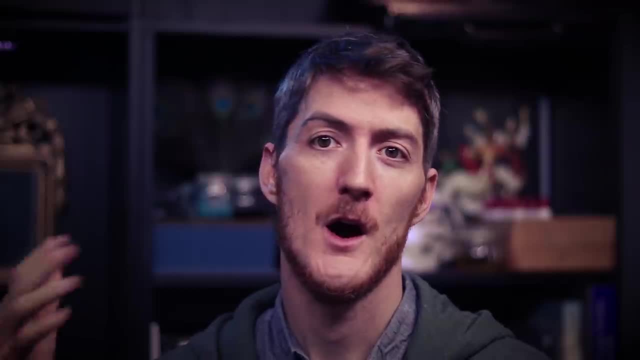 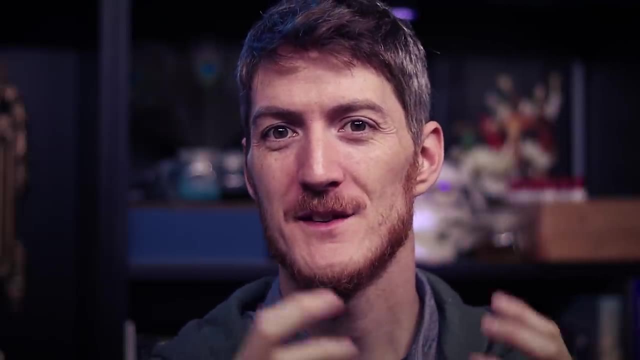 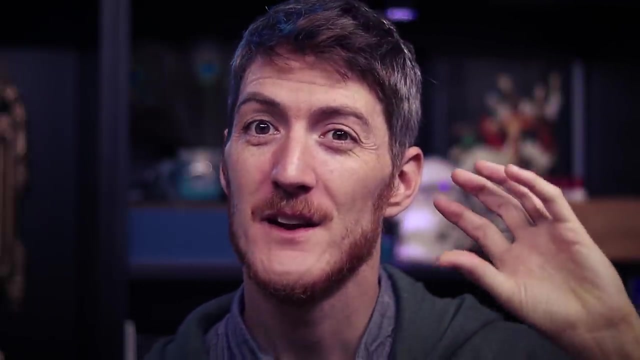 That there could be a harmonic structure of coloring And it doesn't take away the subjective and creative part of the visual arts, It's just having a structure, And that structure helps you find your way and find your approach, find an artistic and creative statement and use colors accordingly. 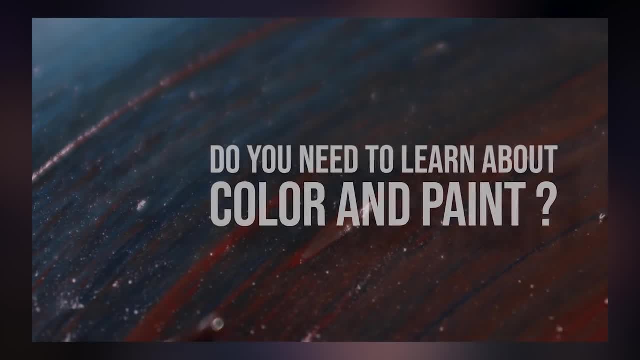 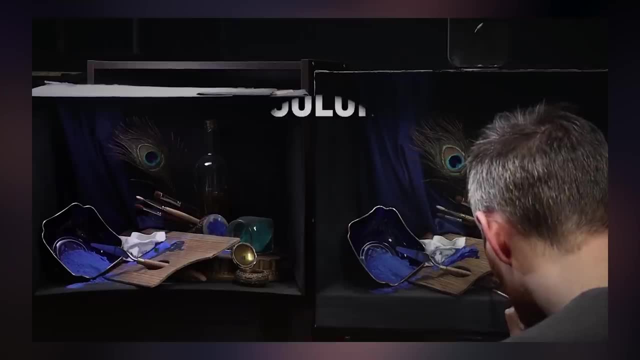 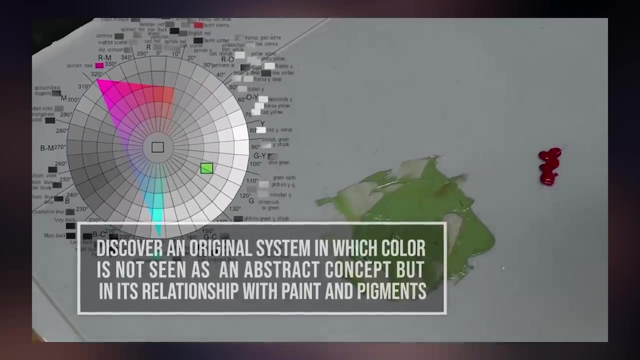 So if you want to explore color and paint further, you can have a look at my new painting course on color and the art and practice of color. It's a nine-hour course focused on color theory and its application for painters. Everything is designed to help artists transpose color knowledge into art. 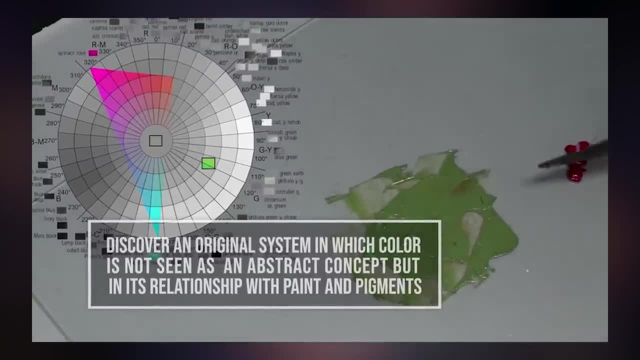 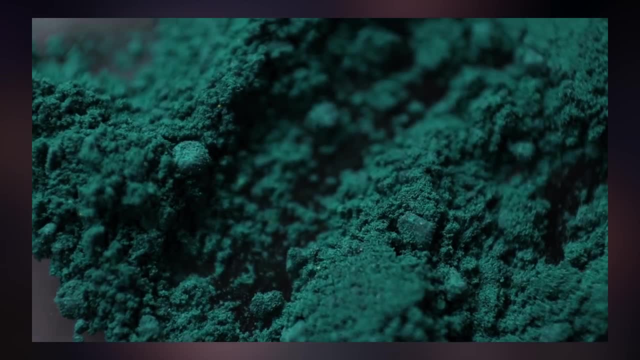 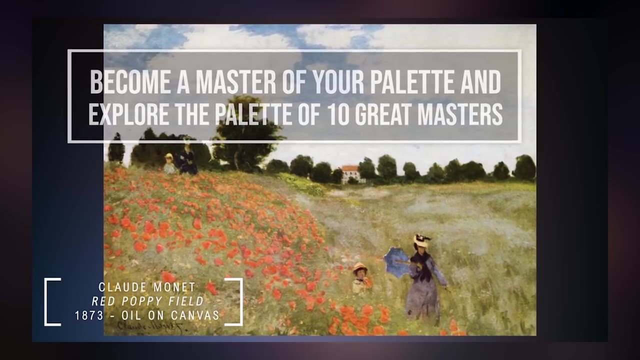 Color wheels, pigments, mixing, transposing colors, color harmony, etc. It contains everything, with three complementary demonstrations: a still life, a landscape and a portrait. If you're interested, you'll find the links in the description. Just have a look, It's a simple click. 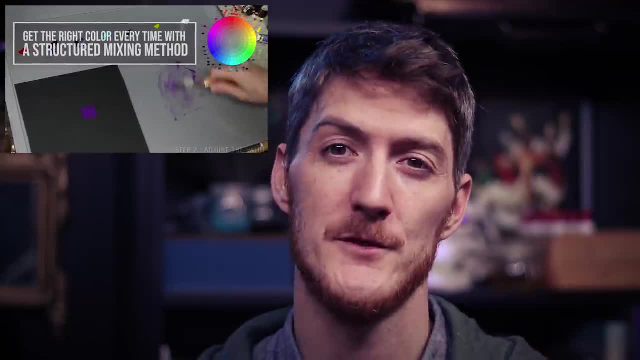 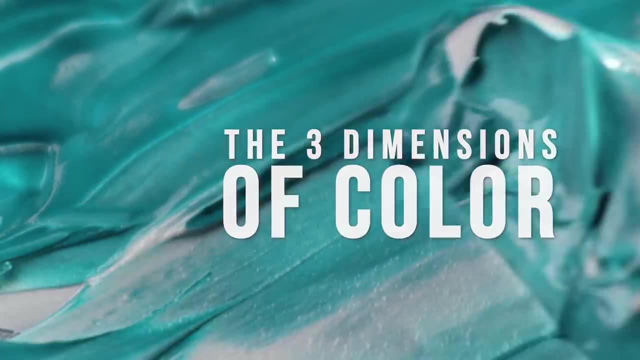 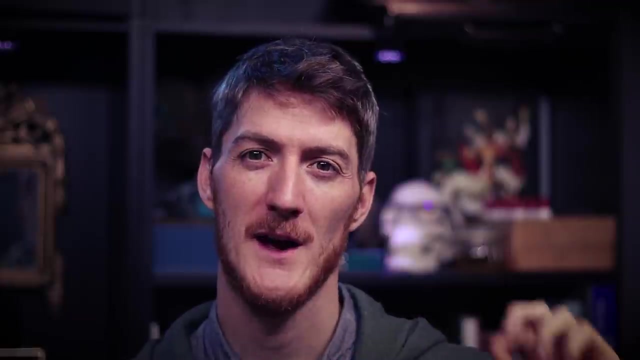 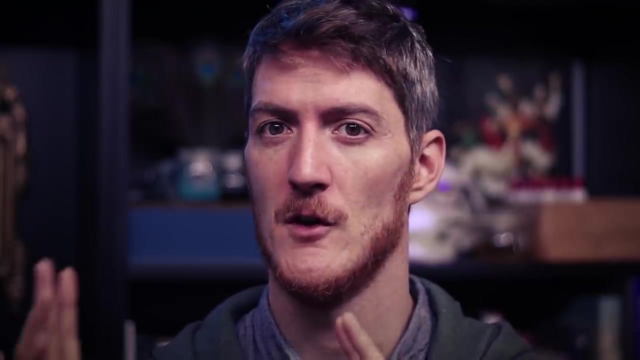 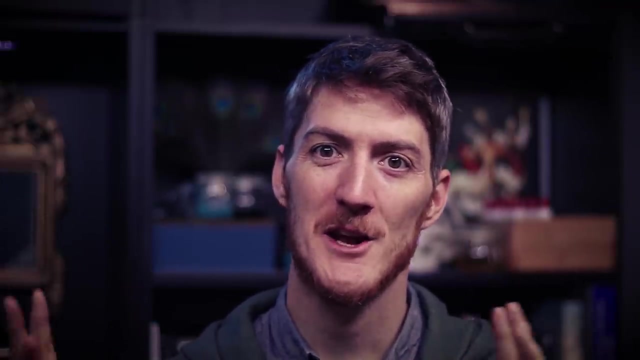 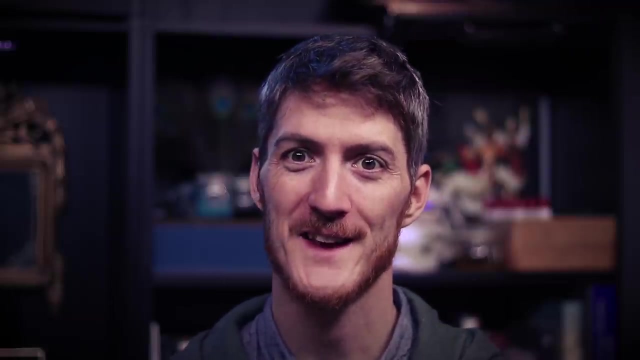 And it's not only great resources for your art, but it also helps the channel tremendously. So thank you for checking out the course. I'll see you next time. Bye, I'm sorry, I'm really wrong, so let's not do that. 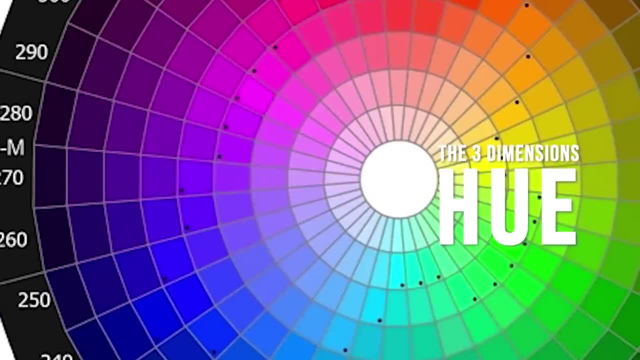 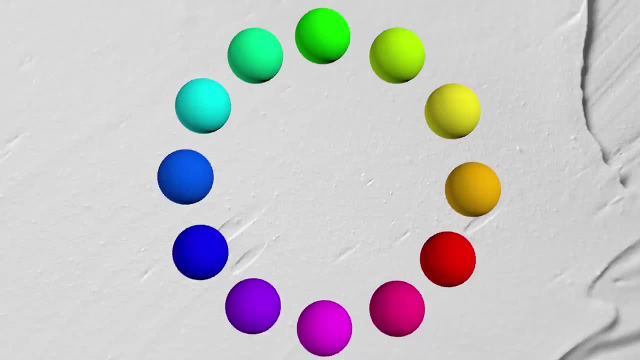 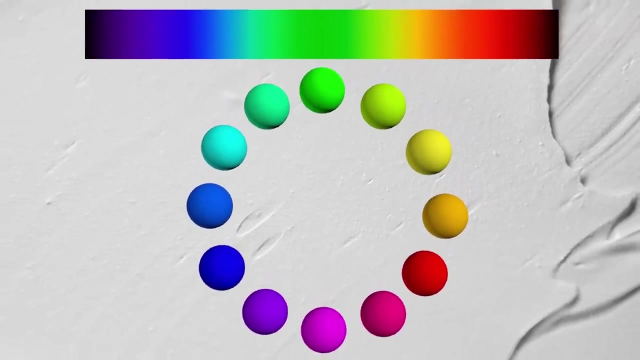 And let's see what they're all about: Hue. So hue is what is commonly referred to as color, but it's just one aspect of it: Red, yellow, orange, blue, purple, and all the constituents of the visible spectrum are hues. 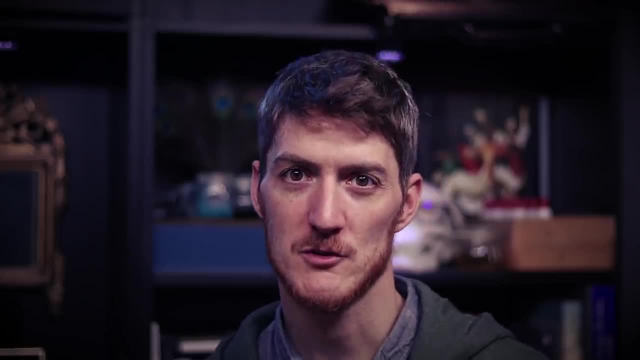 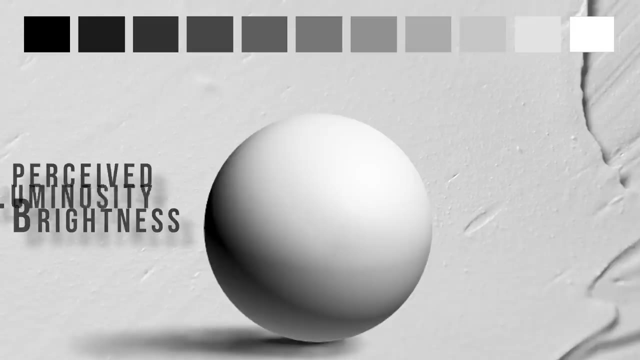 The hue of a color corresponds to the wavelength of light or to the mixture of wavelengths of light Value. The value of a color is its perceived brightness, Sometimes called luminosity. When we say that a color is dark or light, we're actually talking about value. 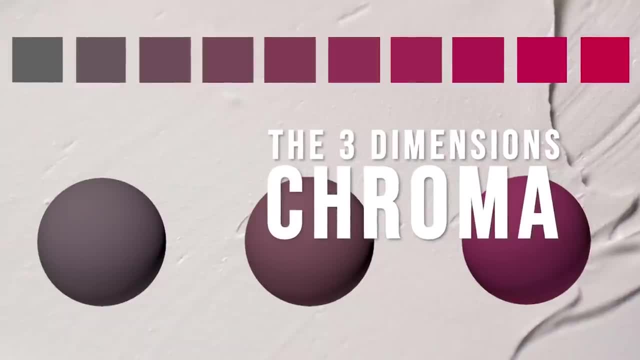 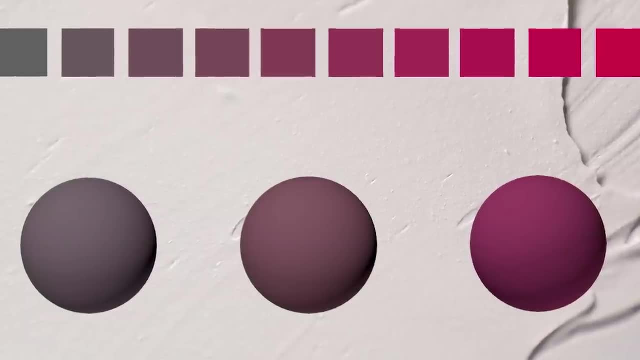 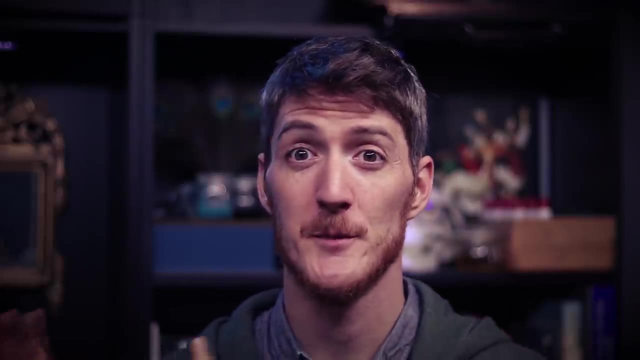 And finally chroma. Chroma is sometimes called saturation. There is actually a technical difference between the two, but given the fact that they sort of represent the same idea, we can consider that they are the same thing. Chroma saturation, or sometimes hue purity, is what makes us say that a color is more or less visible. 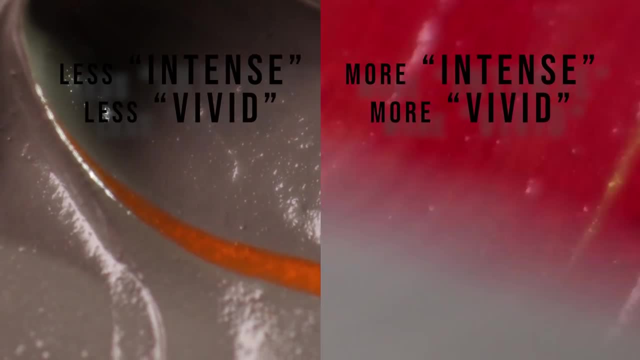 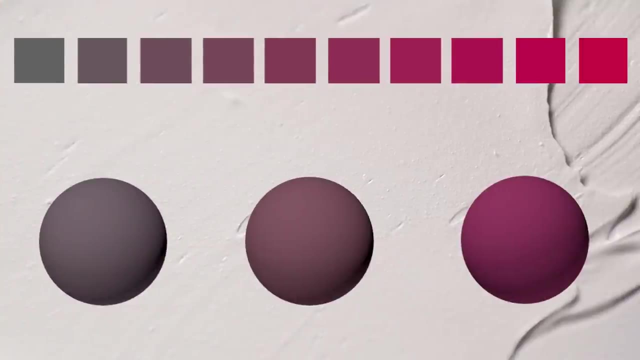 A color is more or less vivid, more or less intense, more or less vibrant. Let's say, this sphere on the left has a low chroma because it's very close to gray, Whereas the sphere on the right has a high chroma because it's a lot more intense. 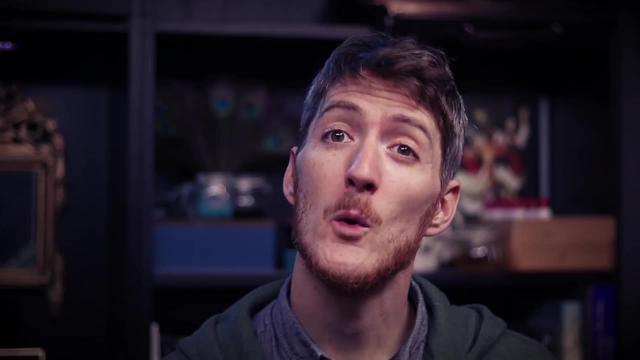 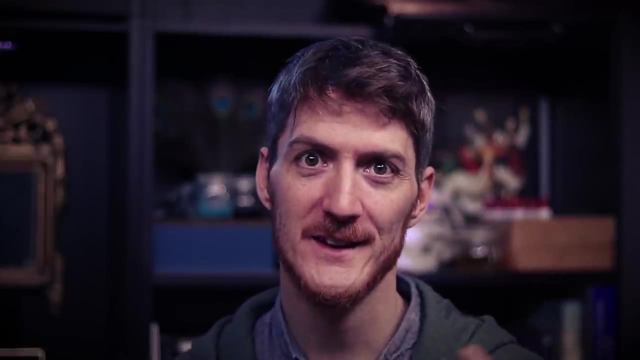 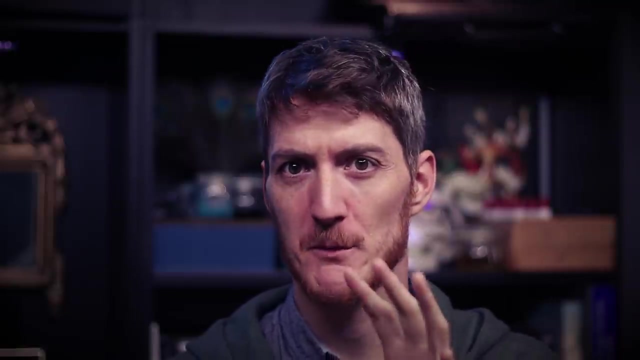 Color theory. Now we need to find a color theory that incorporates all these dimensions of color, And it's not easy. Most of the existing theory forgets at least one dimension, except the Mansell color system, which I can talk about in another video. 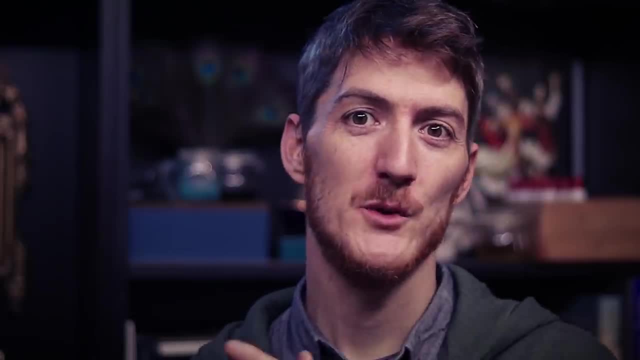 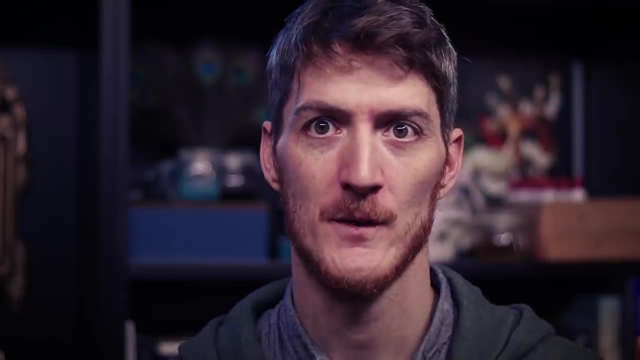 It's a different thing And most of the time, value is left on the side, And it's unfortunate because value is a super important aspect of color. If you don't understand value, it's really really hard to understand lights and shadows. 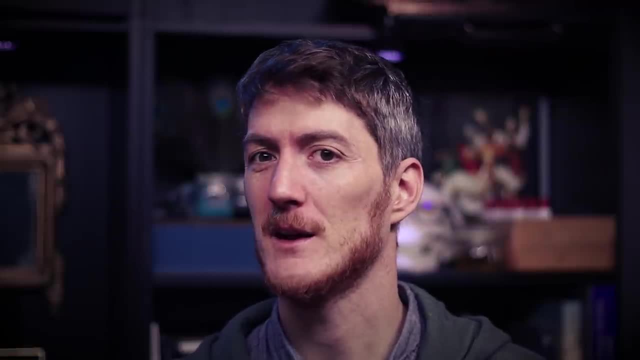 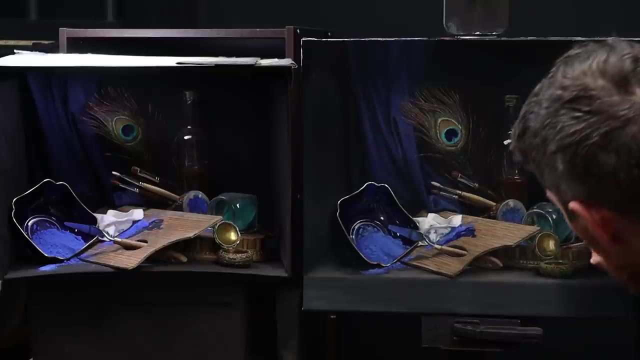 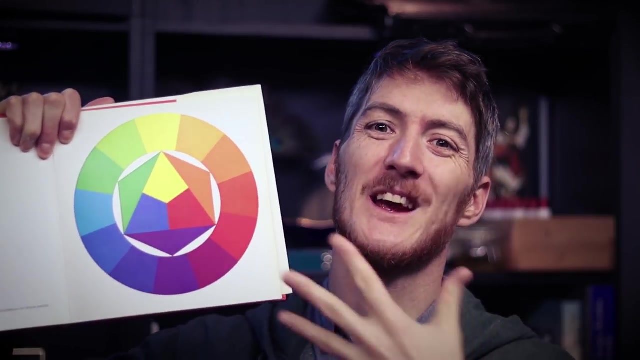 So you end up creating a color theory That's basically not helping you to paint anything in volume, So for figurative painting it's going to be pretty much worthless, All right, So I want to show you the limitations of a color theory that doesn't include all these dimensions of color. 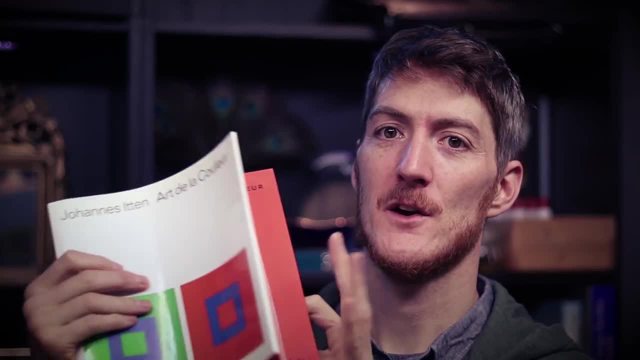 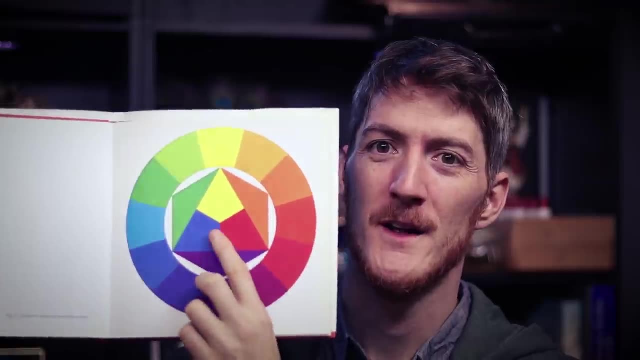 And let me take this example. This is a color theory book written by Johannes Itten. It's a pretty famous book And I'm sure you've seen this representation before. This color wheel is like this. This color wheel is a classic. 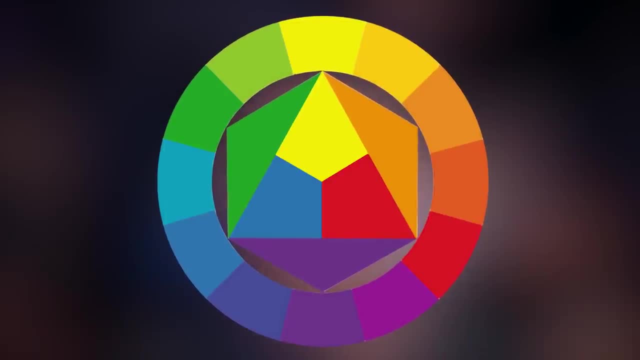 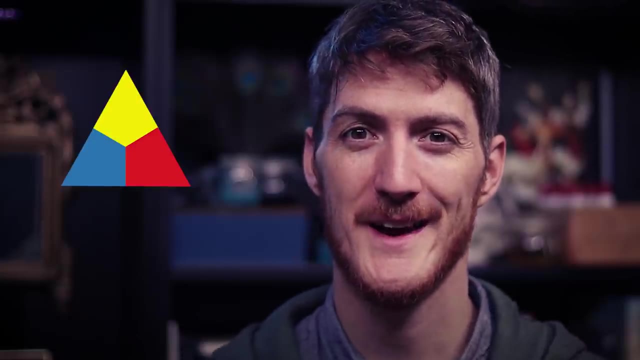 So classic actually that it sort of became a traditional color wheel for color theory. It shows a color wheel organized around the three supposed color primaries red, yellow and blue. So you get the idea right: Red and yellow make orange. 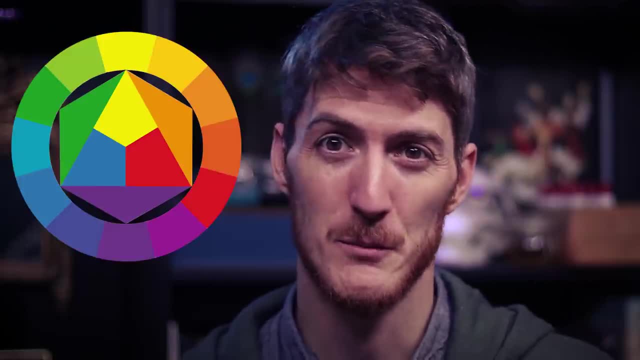 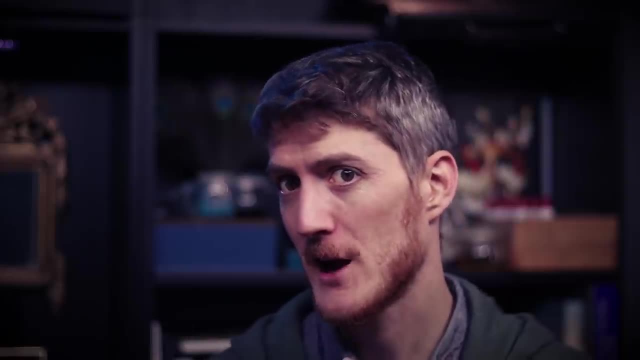 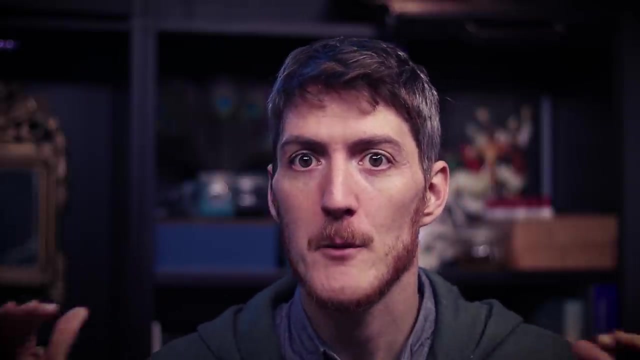 Yellow and blue make green And blue and red make purple. It's a pretty simple theory, Easy to grasp And it's actually decent. It actually does work like this And it's been considered a classic- So classic that it became really primary school level of color theory. 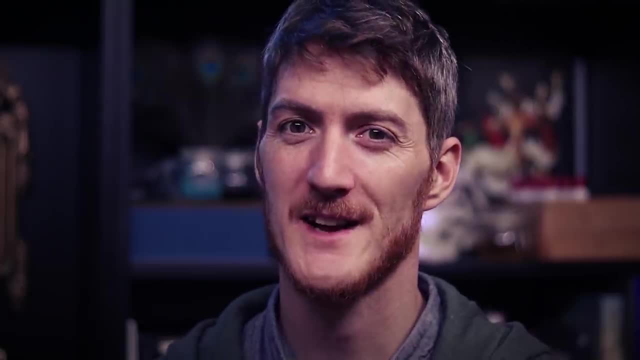 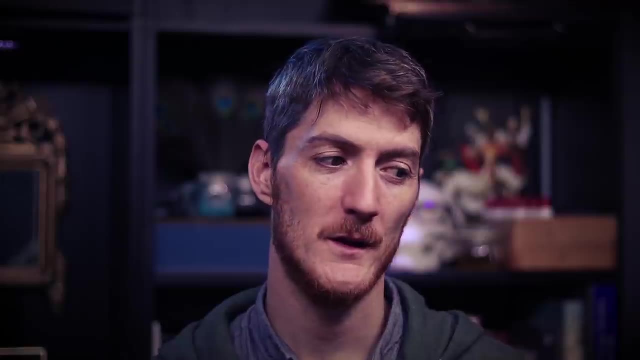 This is what you would learn at school, But for painters it's actually quite limited, And there are actually kind of problems with this model. The first problem with this wheel is, for example, how would you get this color here, Yellow and blue? 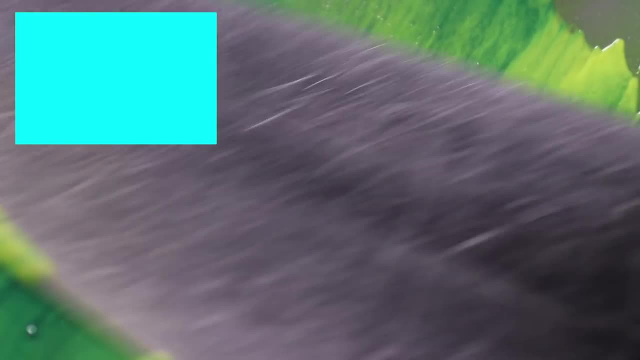 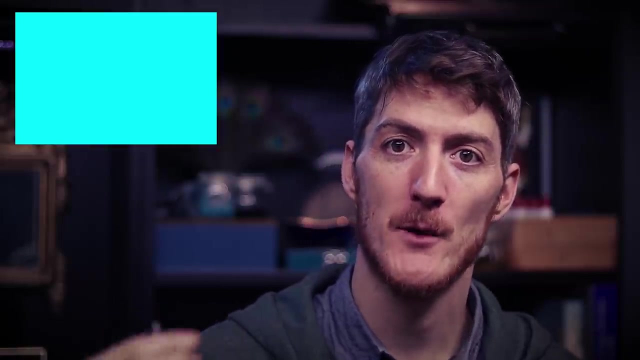 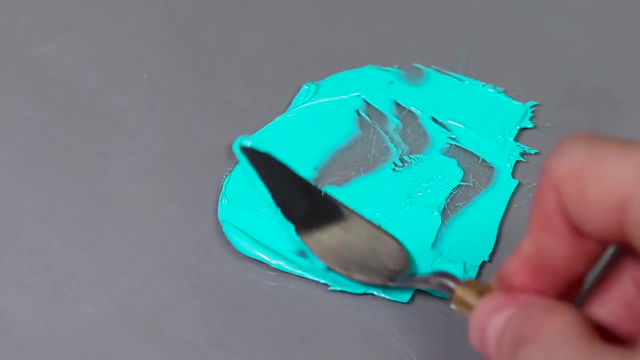 No way you can mix the right color. Not light enough, Not enough chroma. So what you would need to do to mix this color is actually add an extra primary to the color wheel to compensate for this limitation of this wheel. that's just organized around three primary colors. 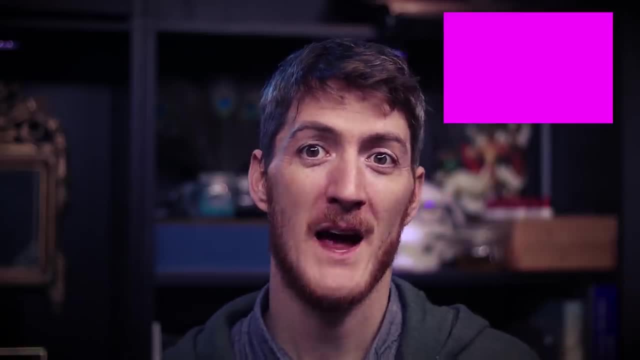 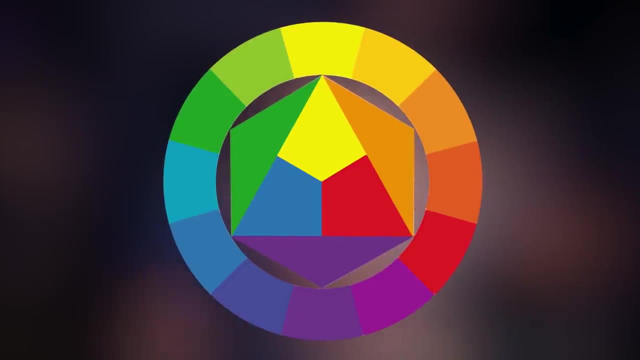 And it's the same thing for this color as well. How do you mix it with this? You have to bring an extra pigment And see. this is the problem with this model- is that it's a deductive model. Everything is derived from this. 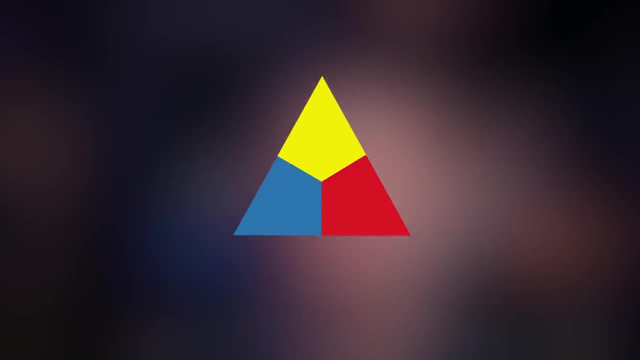 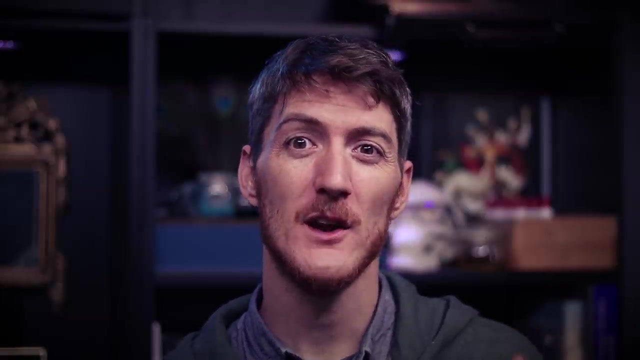 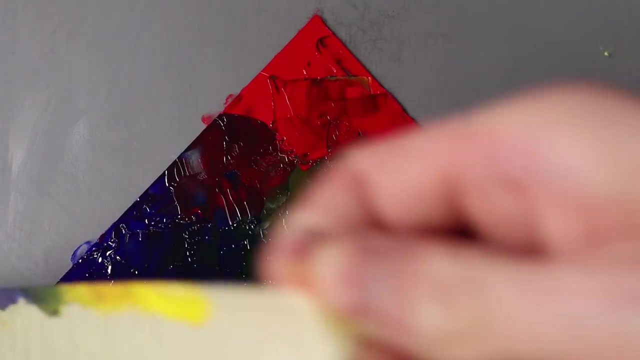 Everything is derived from the three primaries red, yellow and blue. It sounds really cool on paper, but in an actual painting situation you actually need to leave a lot of colors on the side, simply because they are not part of this triangle gamut formed by red, yellow and blue. 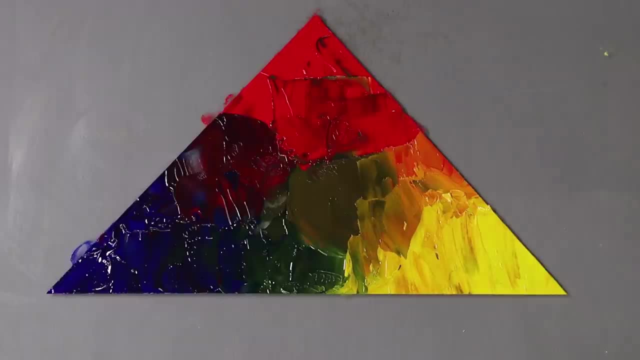 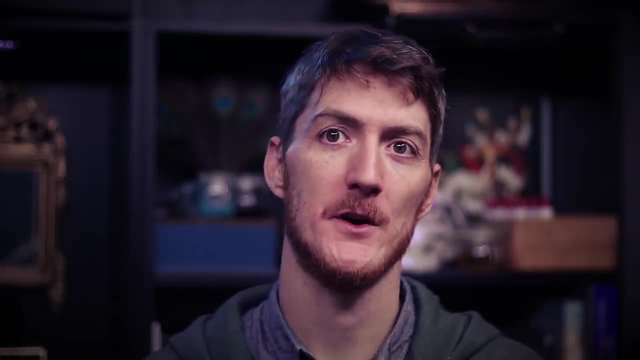 They are outside of this gamut, So you have to bring extra pigment. The second problem is that red, yellow and blue are far from being ideal primary colors. They work in most situations- Don't get me wrong- And you can use them. 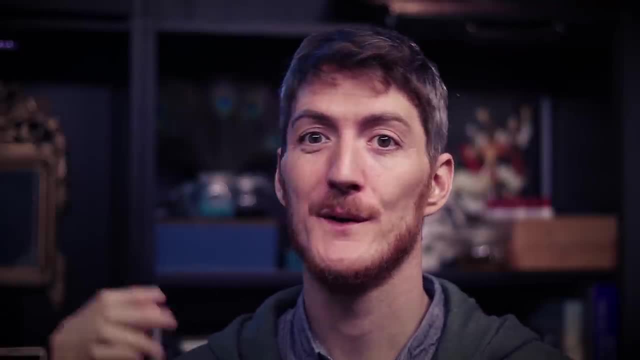 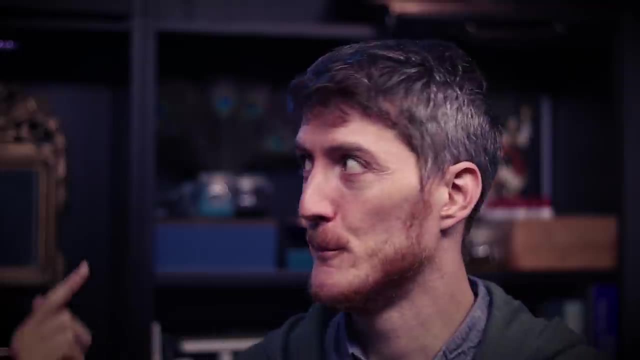 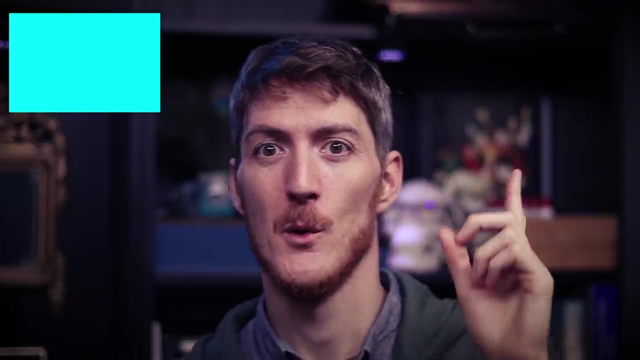 They have really good pigments And you can actually use only red, yellow and blue and achieve realistic colors for most paintings. Why? Because most of the colors around us are actually pretty dull, So you don't need to create this or this. 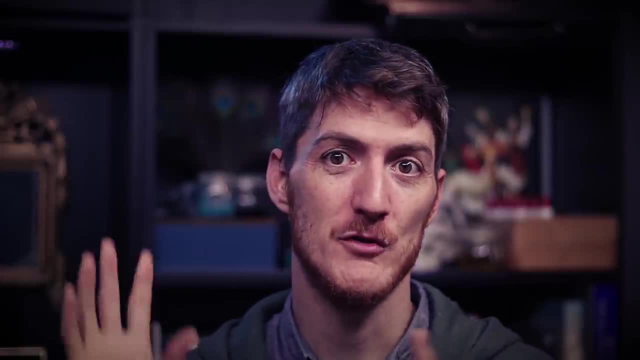 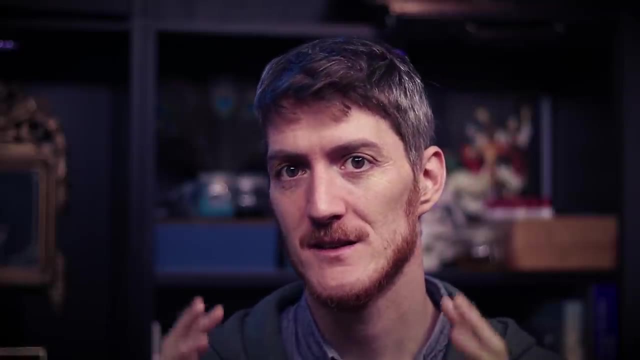 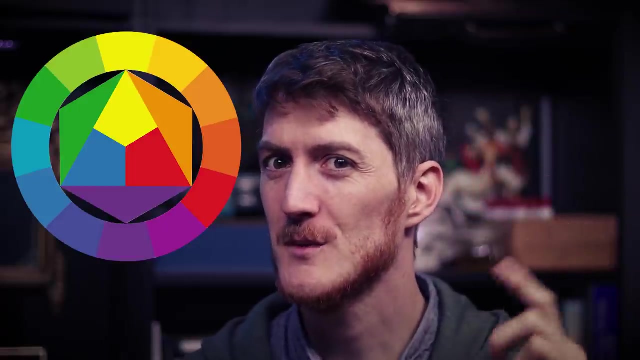 So it's okay if you don't have colors that allow you to make these very rare shades. As long as you can make the dull browns and things like this, it will work. Now, stating that they are the foundation for the entire color system is something else. 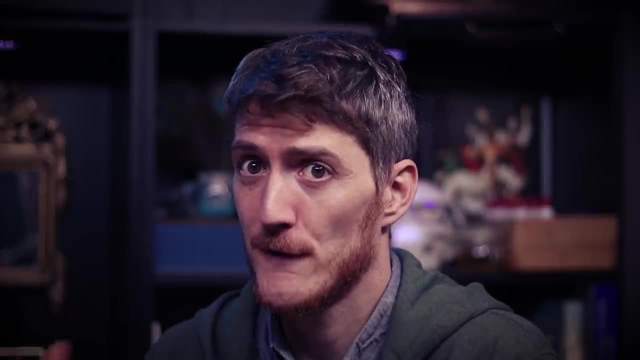 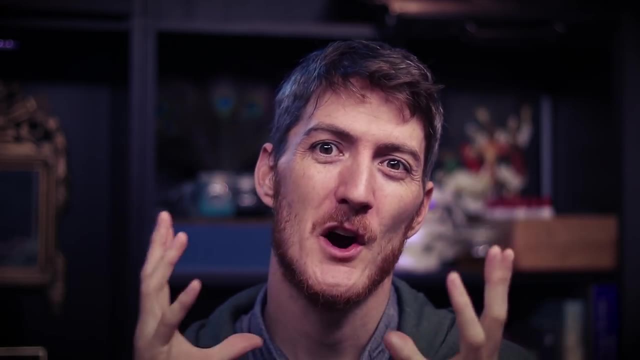 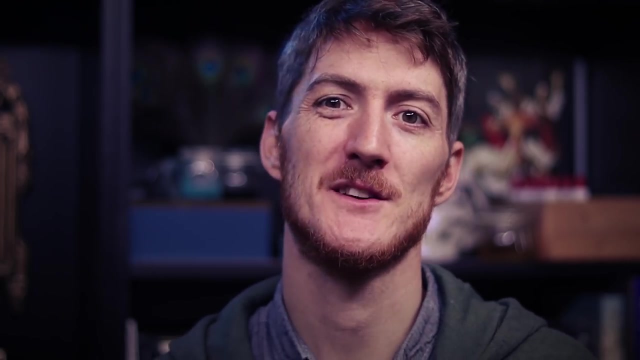 You can use them and practically they work fine and you can paint with them, But saying that they are sort of the roots of an entire color system, it's simply wrong. I mean, the notion of primary color itself is complicated. I'm not going to explain entirely why in this video. 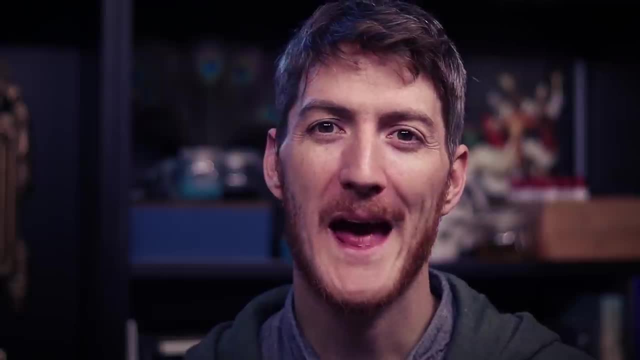 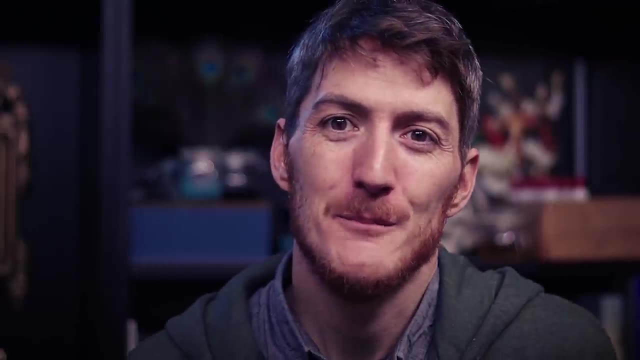 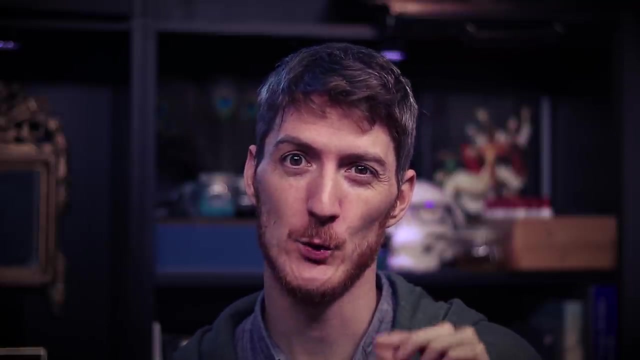 But let's just say that red, yellow and blue as primaries on which we can base an entire color theory, an entire color system, is simply not good enough. The third problem with this system is that the complementary pairs simply don't work. 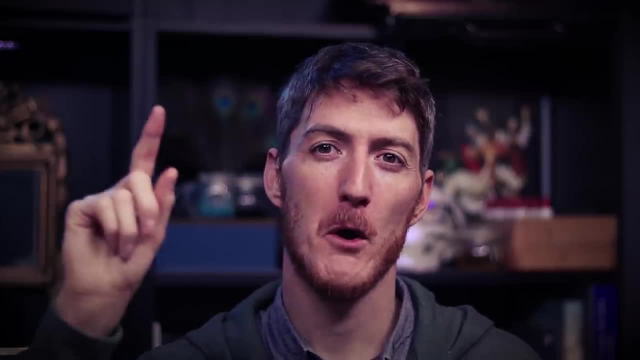 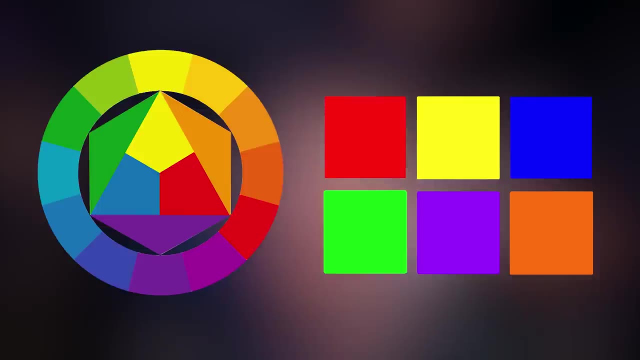 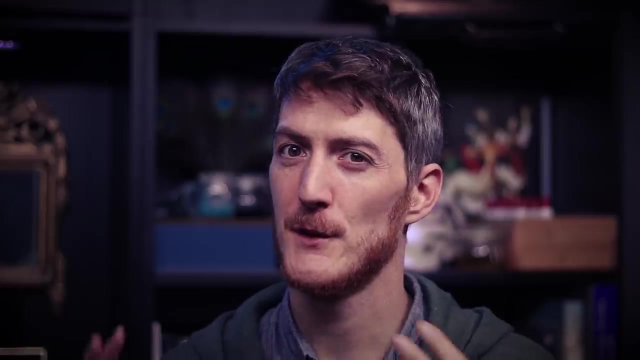 As a reminder, complementary colors are opposed in the color wheel, So normally, if this model was right, we should have red complementary to green, blue complementary to orange and yellow complementary to purple. The thing is, the complementary are not decided randomly like this. 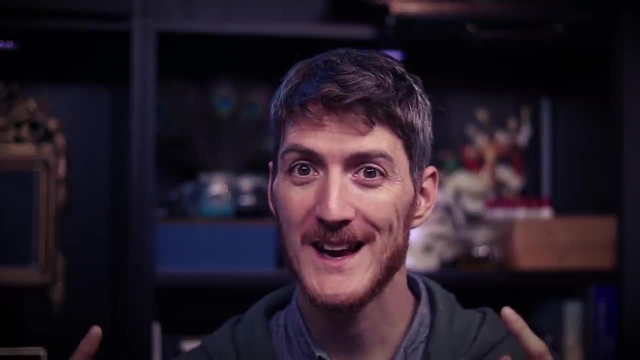 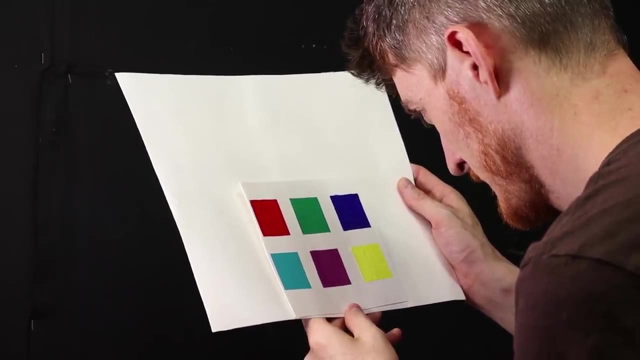 They are actually based on human perception. We can see the visual complementaries by the phenomenon of retinal persistence. So let's have a test. I'm going to ask you to keep your eyes on the little dot in the middle and don't move for 10 seconds. 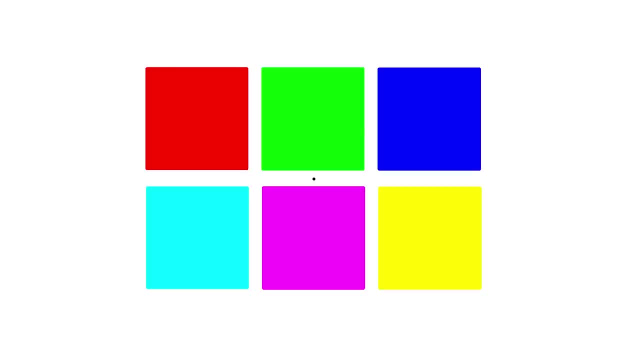 Just don't move your eyes. Stay focused on the dot. The phenomenon of retinal persistence requires you to really keep your eyes still for a while. After a few seconds, the visual complementary of each of these pairs will appear. Are you ready? 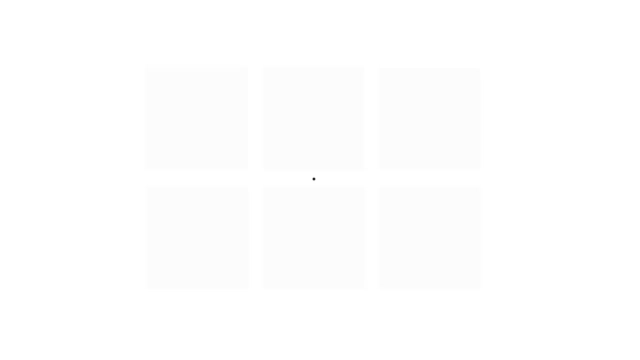 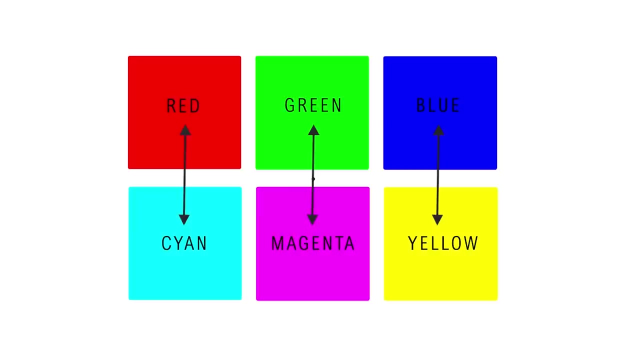 So keep your eye on the dot. Now. you can see that the colors of the squares have been inverted And, based on this phenomenon, we can define the true complementary pairs. Red is complementary to cyan, which is not blue. Blue is complementary to yellow. 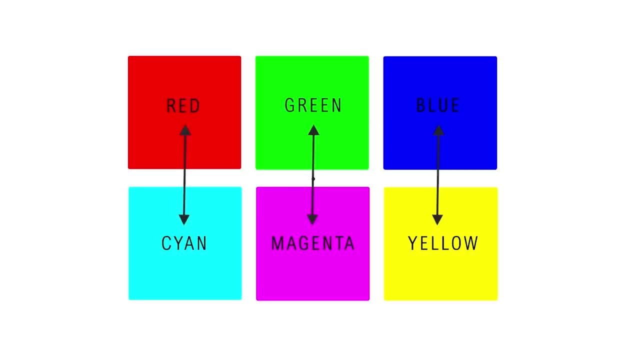 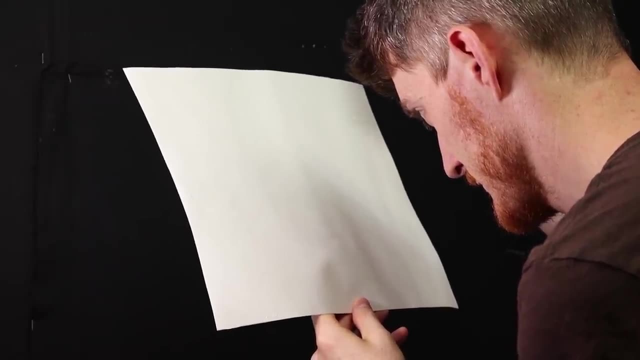 And green is complementary to magenta, which isn't red. If you think that this is an effect of the screen that you're using, you can do the same test with paint on a piece of white paper and you'll have exactly the same results. 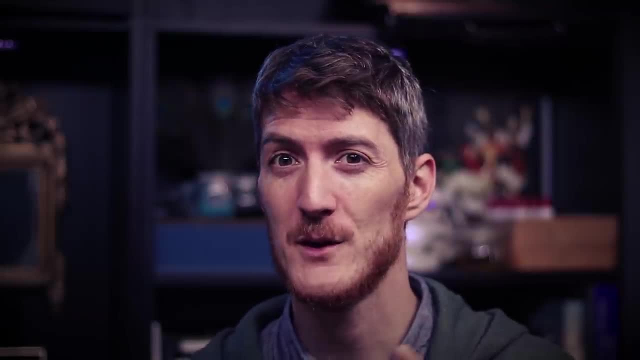 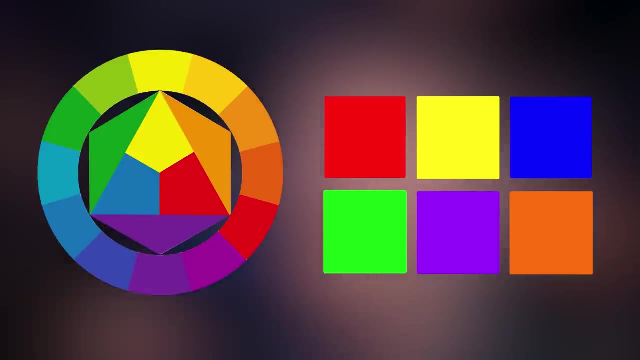 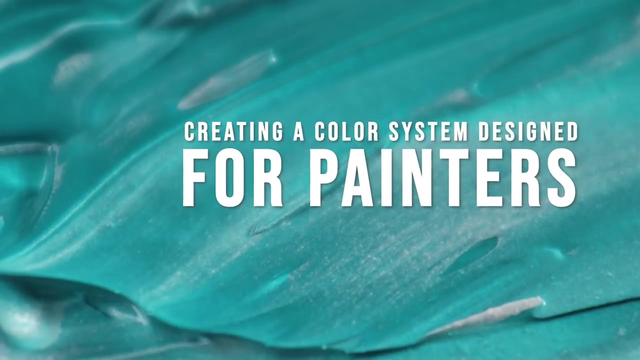 This is based on visual perception. Now you can see that, with this in mind, the color wheel of Johannes Eton simply doesn't work. Red isn't complementary to green, and so on. It simply doesn't work, Okay. so, after this lengthy critique, 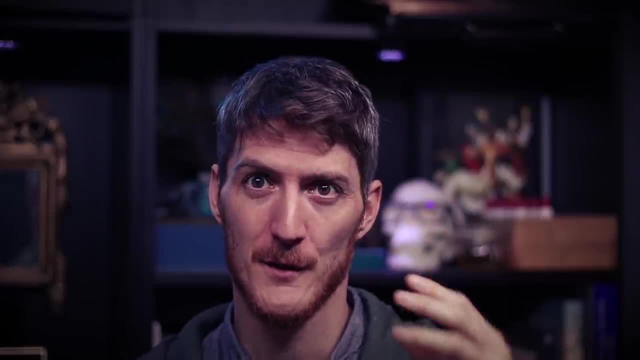 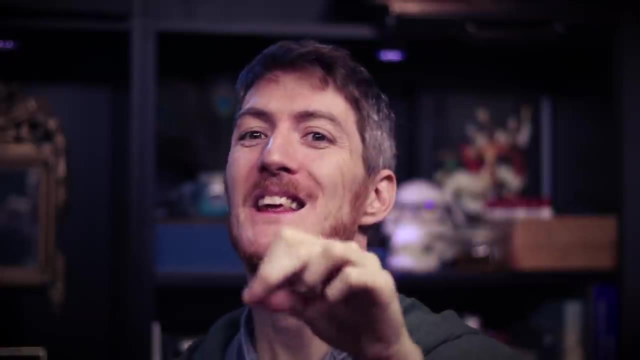 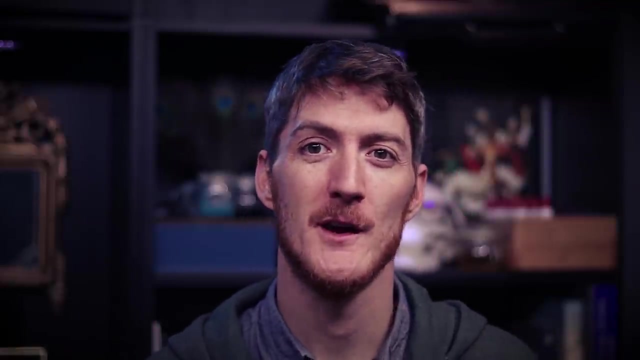 of the traditional color wheel. what can we do? The problem is that we don't want to replace an abstraction that doesn't work with something even more abstract. We have to keep in mind that color theory is only good if it helps us to paint in reality. 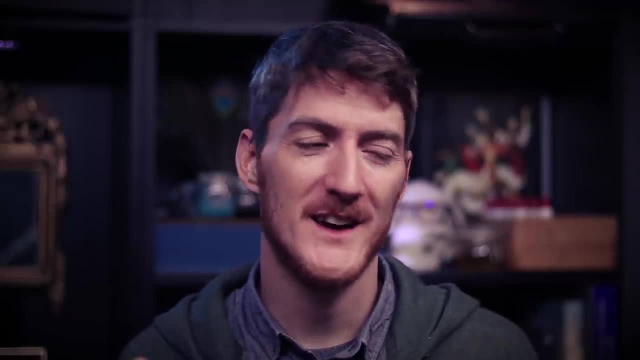 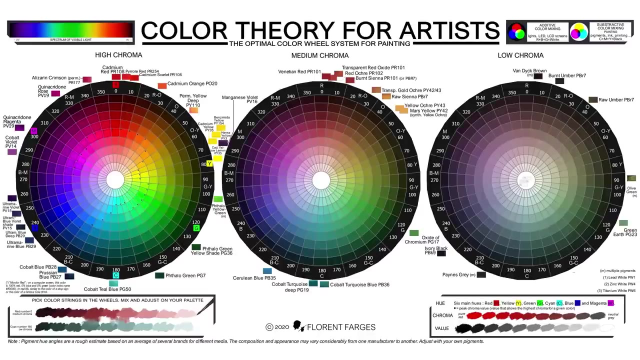 We don't want to enter a speculative fight about color, as if color was something abstract. So let me show you the color system that I've created as a response to this problem, and I'll explain it as I go. I've also created a poster. 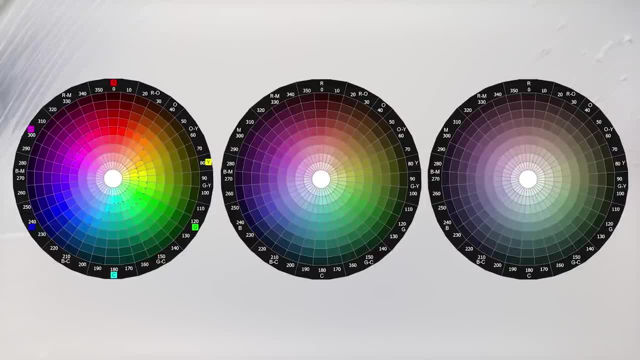 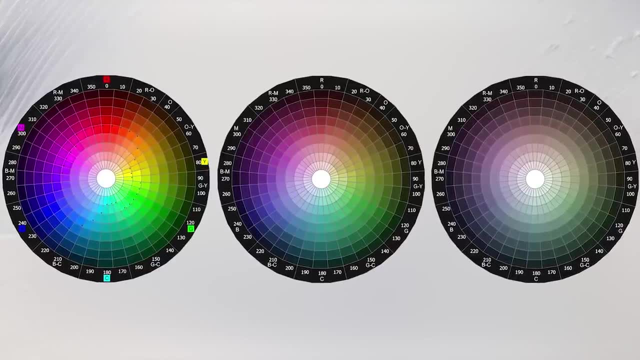 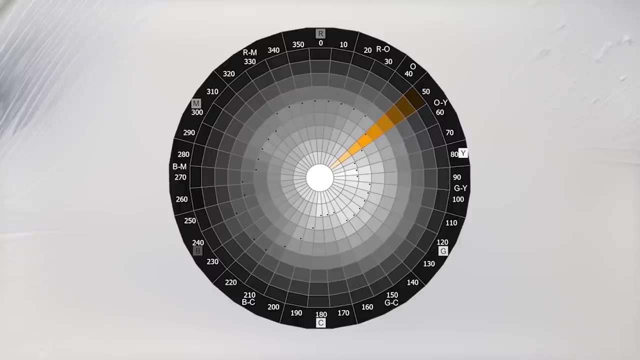 you can find the link in the description box. So when I created this color system, I had three principles in mind. One: I knew that our theory has to describe the three dimensions of color: hue, value and chroma. Here's what I did. 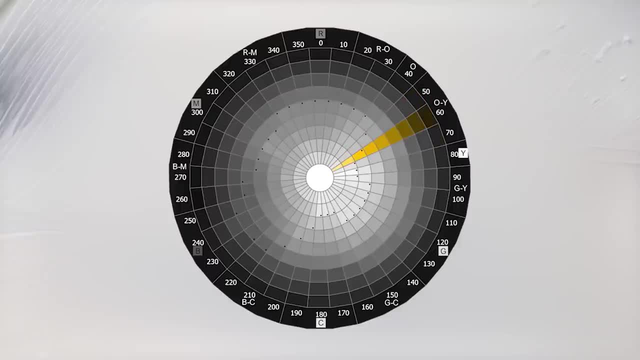 The hues are distributed around the 360 degrees of the wheel. Actually, there are 36 hues, with six main hues- and I don't call them primaries: Red, yellow, green, cyan, blue and magenta. They are evenly distributed around the wheel. 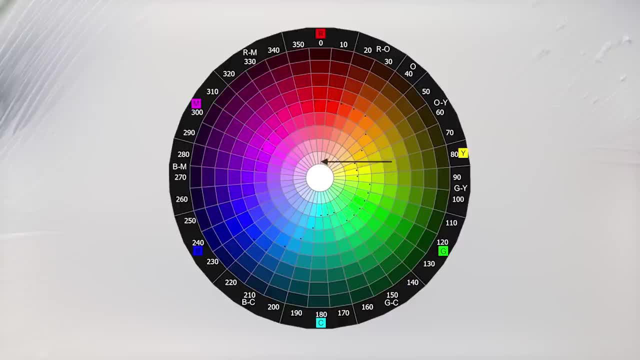 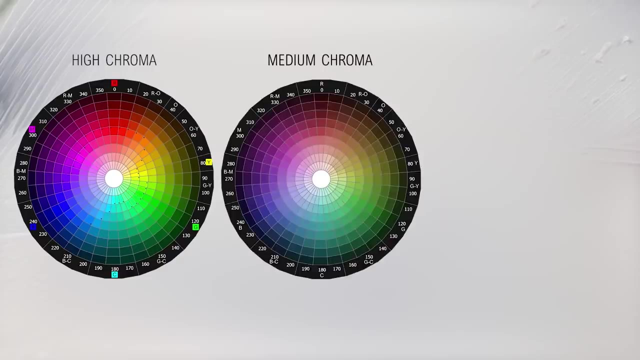 to match human perception. The values are here too. Each hue is part of a value scale ranging from the lightest in the center to the darkest. And finally, the third dimension, chroma, is presented with three wheels. The first show high chroma colors. 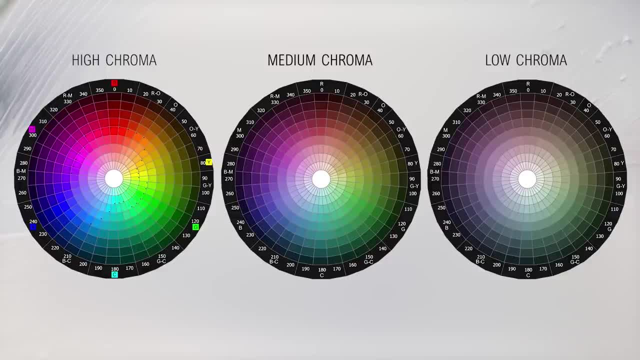 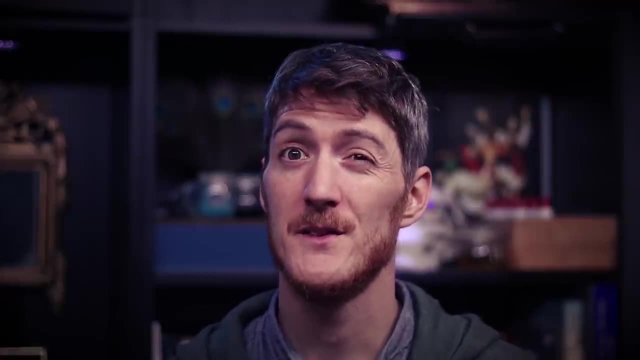 the second, medium chroma and the last one, low chroma colors, And this is how I managed to include the three dimensions of color on a single flat picture. The second principle I had in mind was practical. Our system has to be designed for painters. 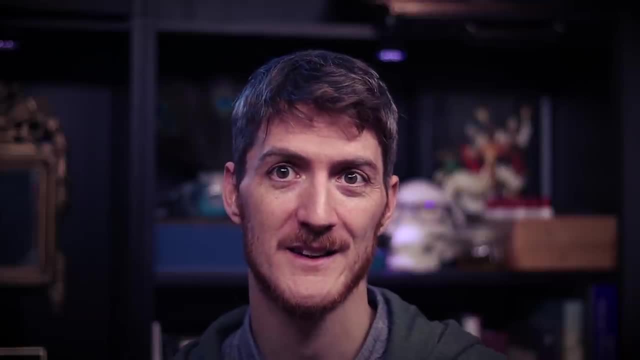 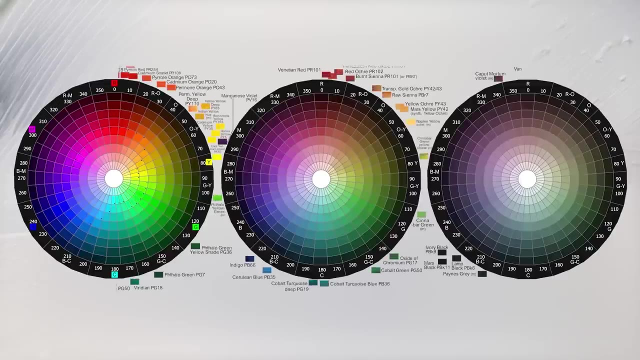 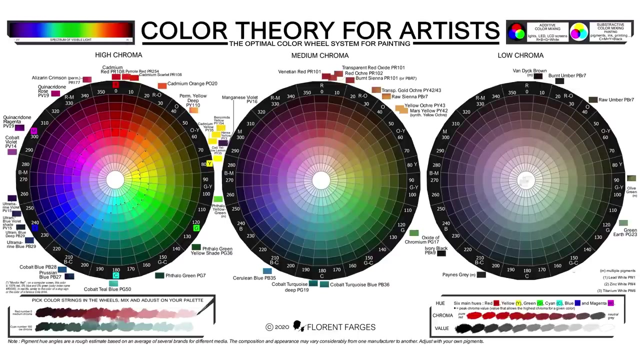 and painters don't use colors. they use paint. So I knew that my color system had to connect pigments and color. Here, of course, there is a lot of approximation, because pigments can vary a lot from one manufacturer to the other, But still. 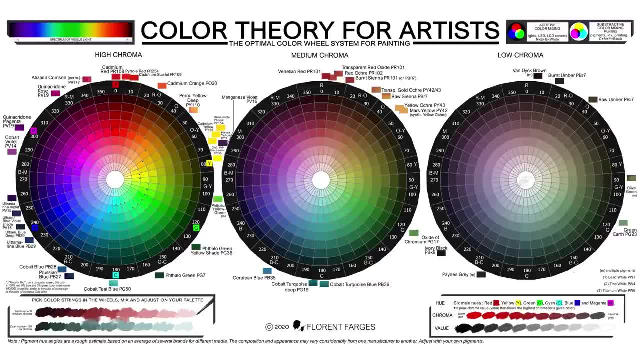 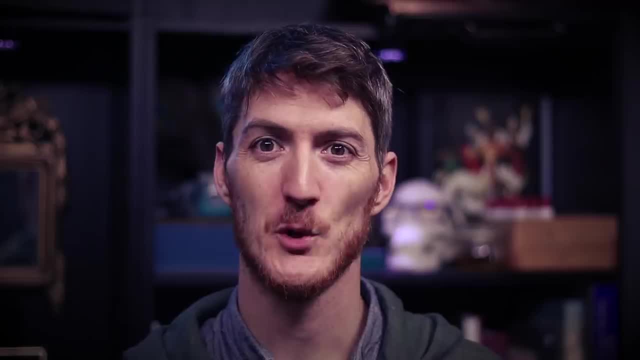 I wanted to show where pigments are located around the wheel to make this picture more concrete. The most important is not the exact placement of each pigment, but the relative placement of one pigment compared to another. So with this color system, you can select the pigments. 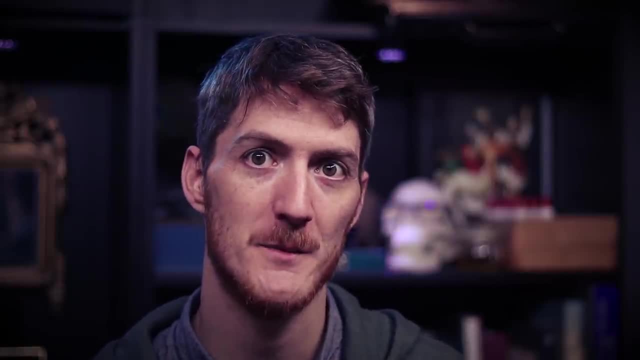 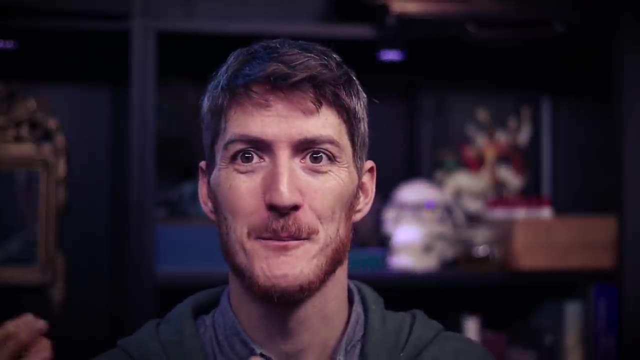 that will work the best for the project that you have in mind. You don't have to stick to red, yellow and blue. Well, you can use them if you want, because they work really well, But if you want to explore other colors, 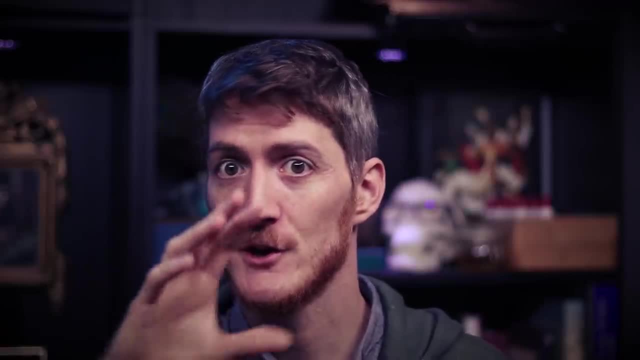 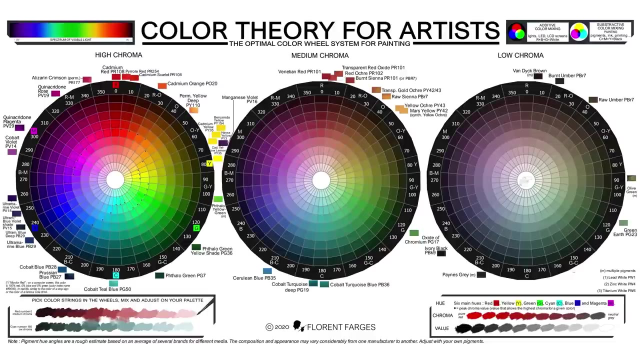 if you want to explore the magenta range, the green range, you are free to do so and you will know which pigments could help you do that. Hopefully, you'll see that the potential is actually limitless if you allow yourself to not be limited by only three pigments. 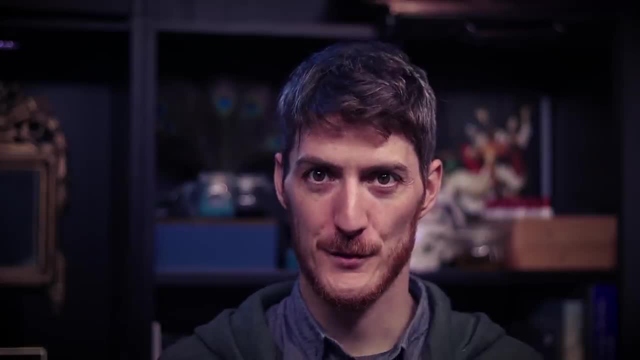 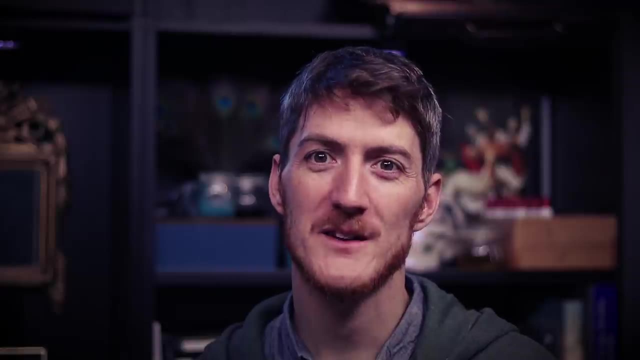 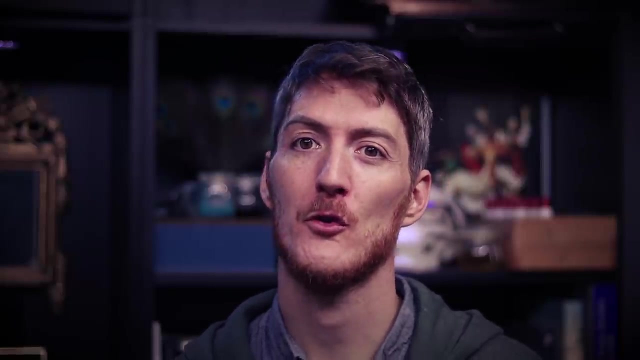 And I hope that this color wheel will help you do that. The third and final principle I had in mind when creating this color system was to make it a practical and an actual mixing tool you can have next to your palette to help you mix, to help you create. 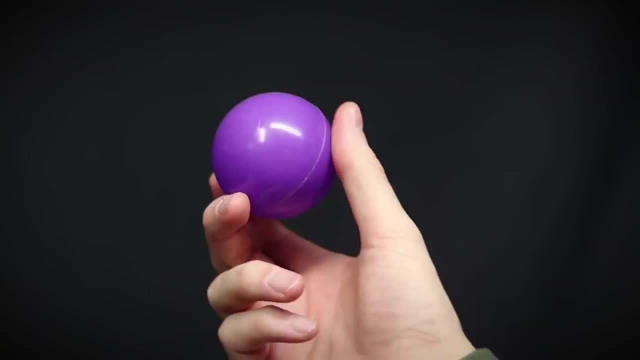 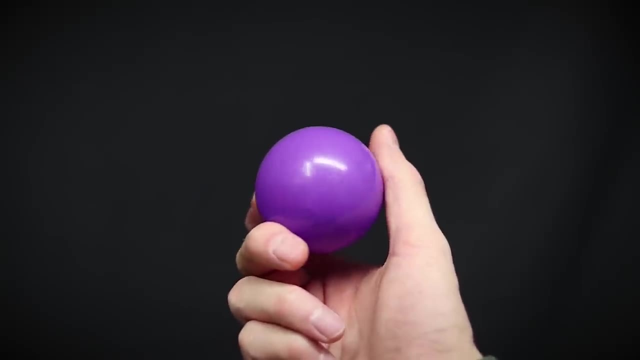 the colors for your paintings. So here is how it works. Let's say that we need to paint this purple wall right here. The first thing to do is to find a couple of candidate pigments. Now there are two options here. One: you have your go-to palette. 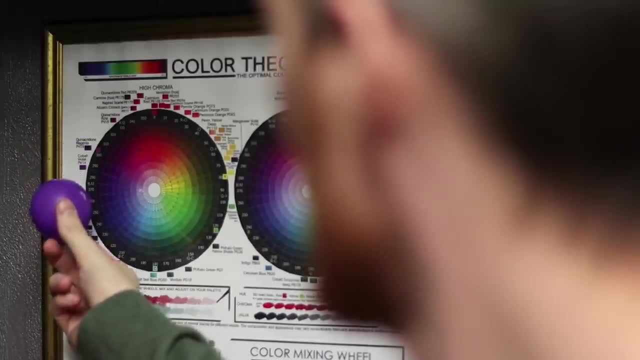 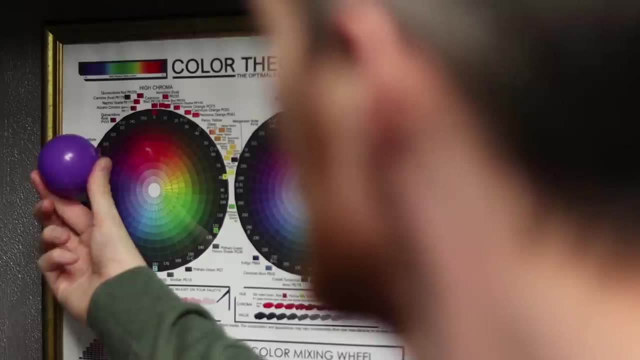 and your favorite pigments that you use all the time, Or two. you will select pigments depending on the type of subject that you need to paint. With this second option, I would need to pick the pigments that are the closest to the colors of this year. 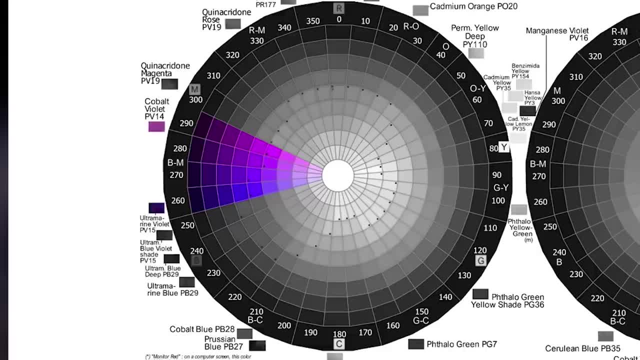 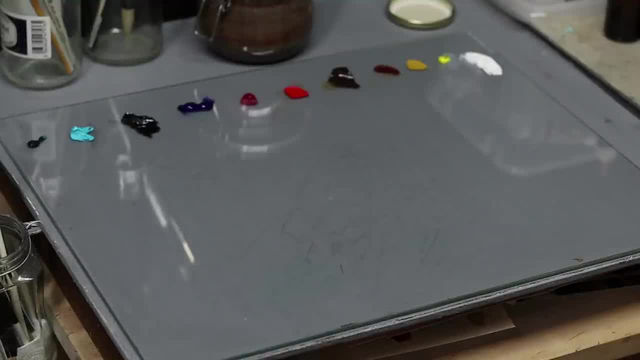 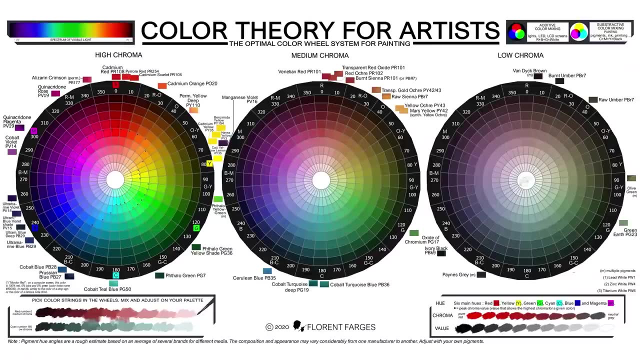 Here I think it would be Cobalt Violet- PV14, or maybe Ultramarine Violet- PV15.. But let's say that we are using our ordinary palette with no violet pigment. Let's say that we can only use the two closest pigments we can find. 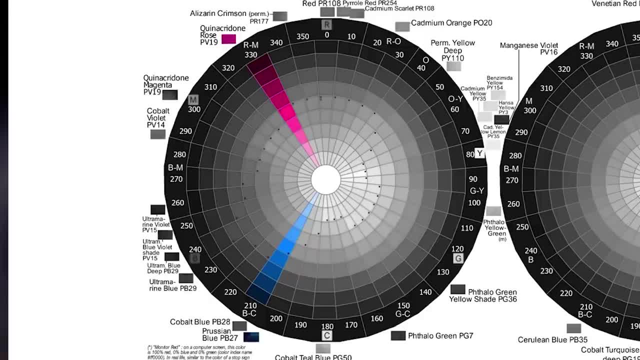 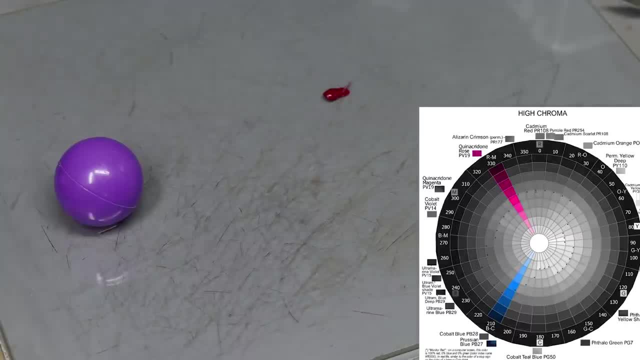 In this case. let's say we have Quinacridone Rose and Prussian Blue. All right, Let's go for that. By navigating the color wheel I see that by mixing those two pigments theoretically I can get the purple. 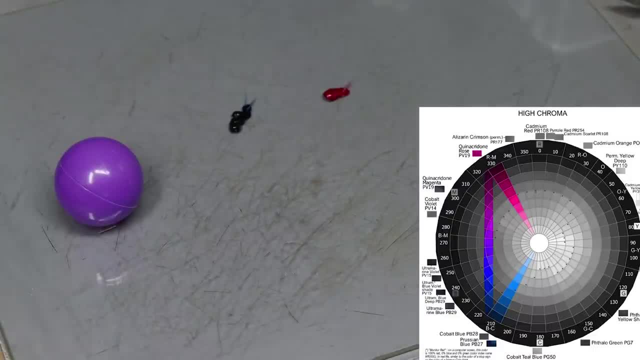 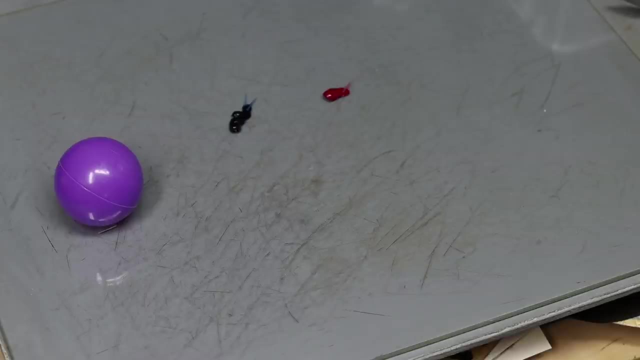 that I need to paint the sphere. So let's try With pigments. you don't really have a choice. You need to try first and see how they react. Don't forget that we are talking about actual substances here with specific chemical and physical properties. 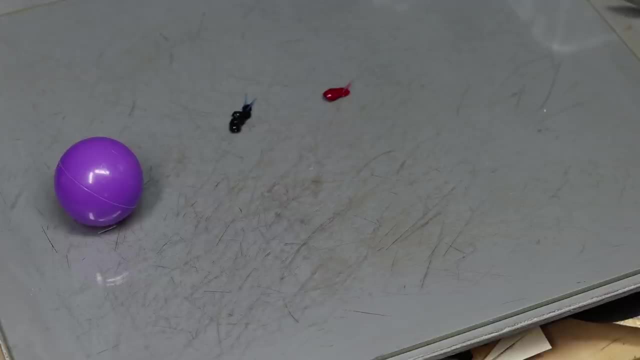 And also that the same pigments can be very different from one brand to the other. There can be a huge difference between what the theory predicts and the result that the real pigments produce. All right, So let's start mixing. Do you remember when I was talking? 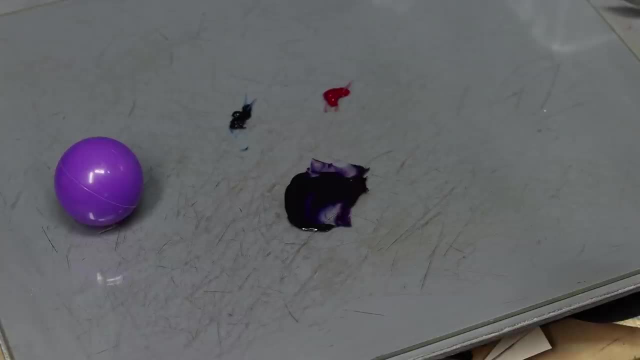 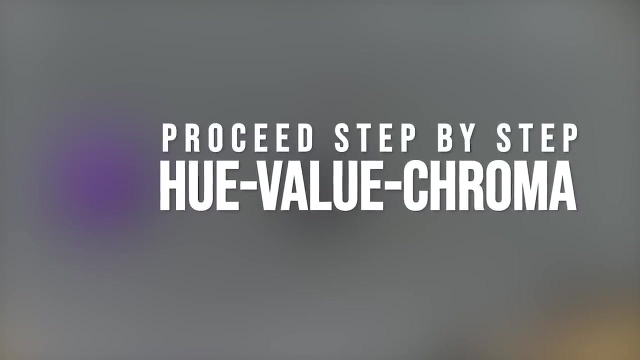 about hue, value and chroma. Well, there is an order to follow if we want to get the right color easily: First hue, Then value And finally chroma. Hey, voluptuous color H, V, C. 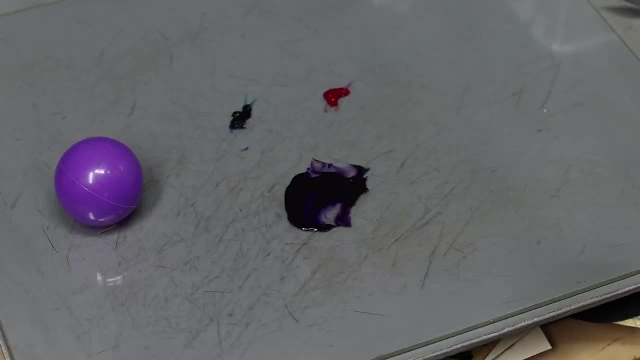 Hue value chroma. That's my mnemonic trick to remember the order. So first hue. I mix Prussian Blue and Quinacridone Rose in equal proportion, first to see what it looks like. Of course, here it's way too dark. 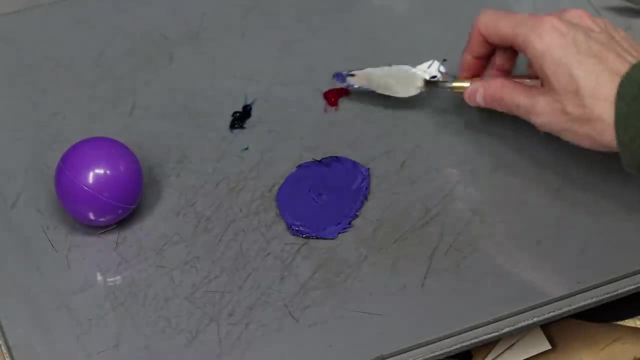 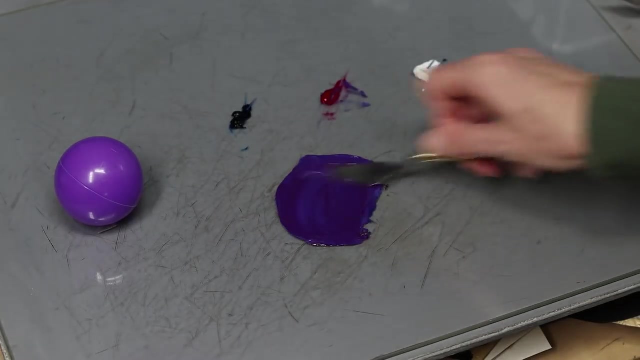 so I add some white to get closer to my target color. I can see that the result is too much on the blue side, so what I'll do is add some more Quinacridone Rose to pull it in the opposite direction If I add too much Rose. 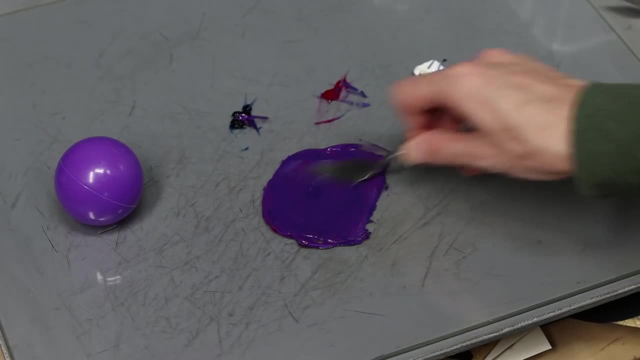 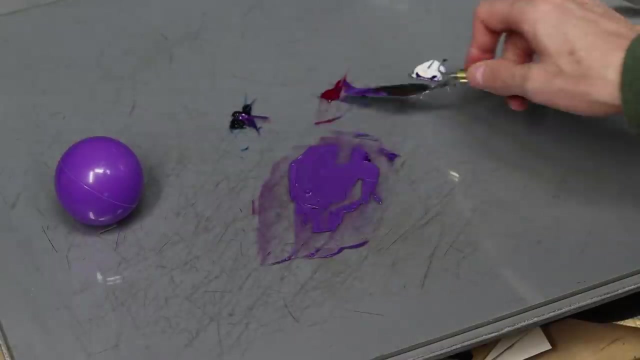 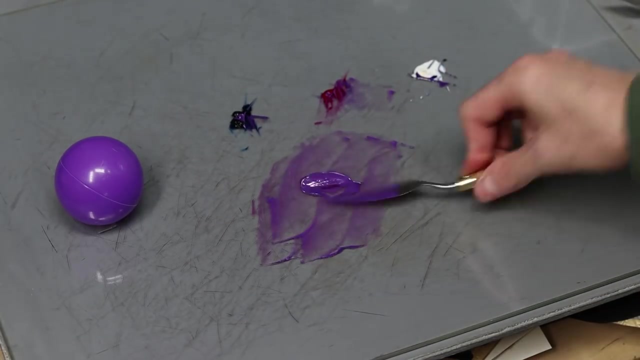 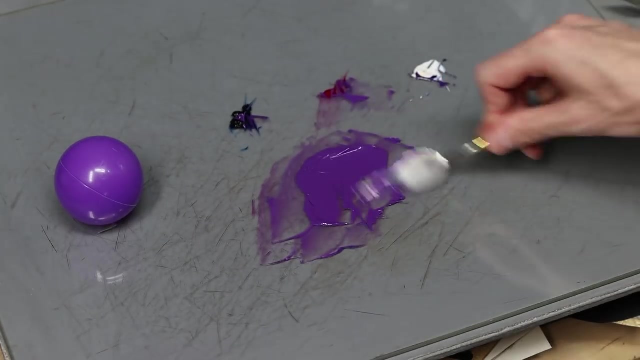 I need to balance again with more Prussian Blue And by doing this with trial and error, with subtle adjustments, I create a hue. that's exactly what I need for the sphere 메이크업 VALUE Once I'm done with hue. 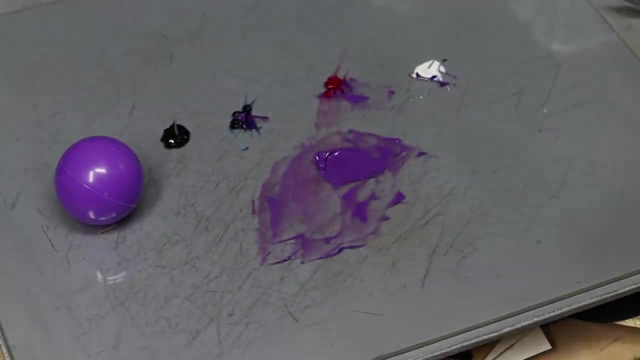 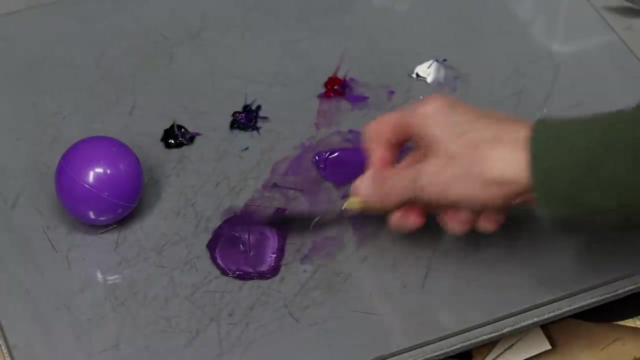 I can make the highlights and shadows. I add Ivory Black and I mix it with Prussian Blue and Quinacridone Rose, those darker shades in the shadows. I don't use only black. I adjust with other pigments and try to keep the character of the shadows. It's not just about 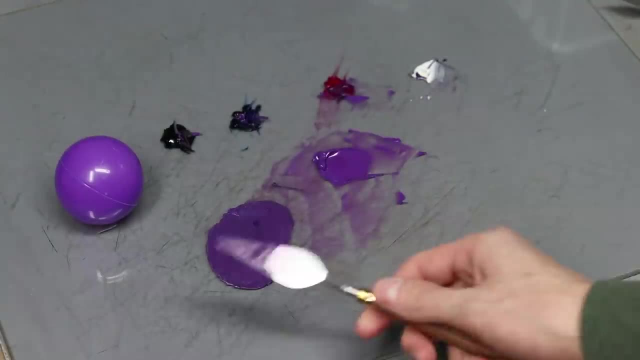 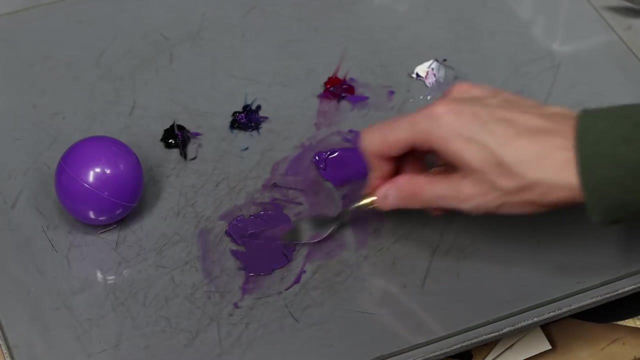 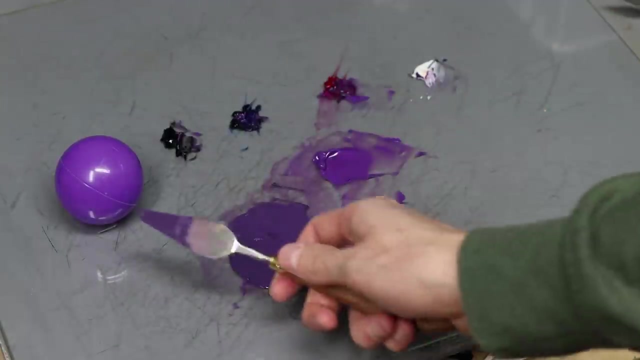 adding black. it's about balancing the dark elements of black with Prussian blue and crunaculum rose. I'm going to make three mixtures, but if you want, you can create the entire value scale and the color wheel can help you do that. 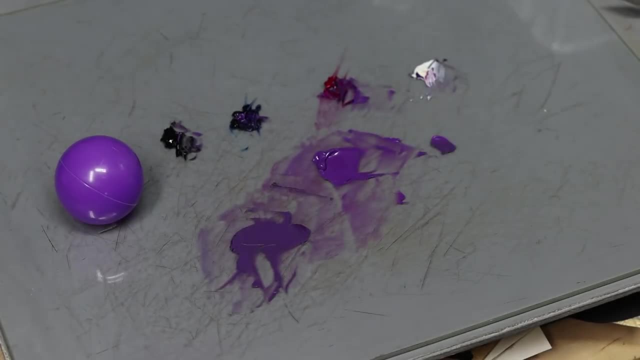 The final thing to adjust is the chroma, because during mixing the chroma can go out of control, so it's important to verify that everything looks fine before painting. In this case, Prussian blue and crunaculum rose can make the chroma. 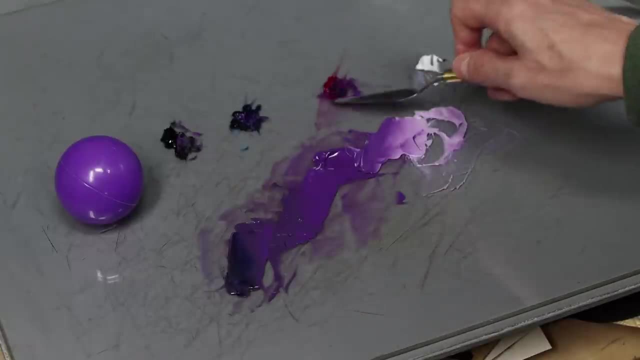 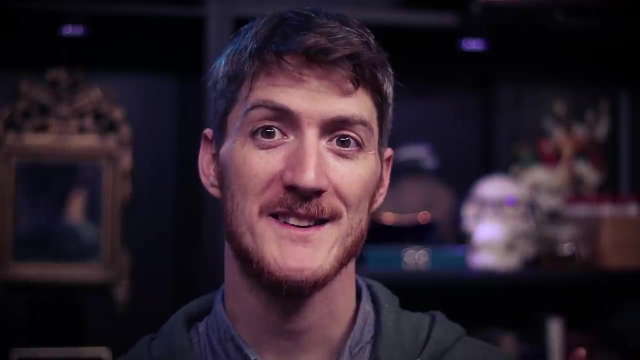 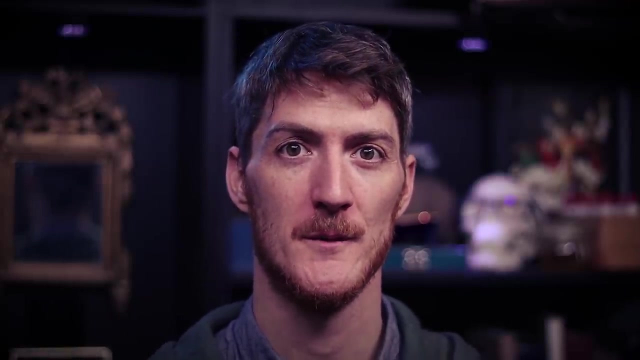 higher because they have a high chroma, whereas black and white will lower it considerably in the color wheel. And that's it now. the only thing left to do is paint. but you see how easy and fluid the entire process was. That's what color theory is supposed to be. It's supposed. 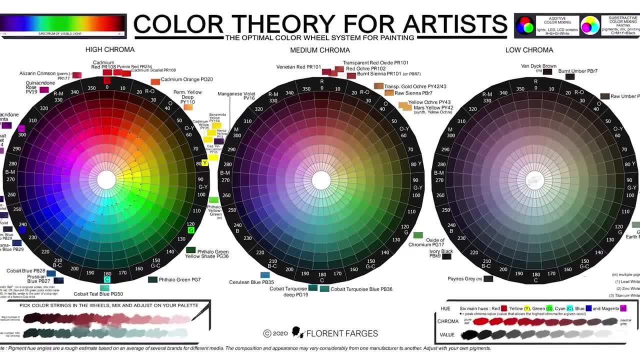 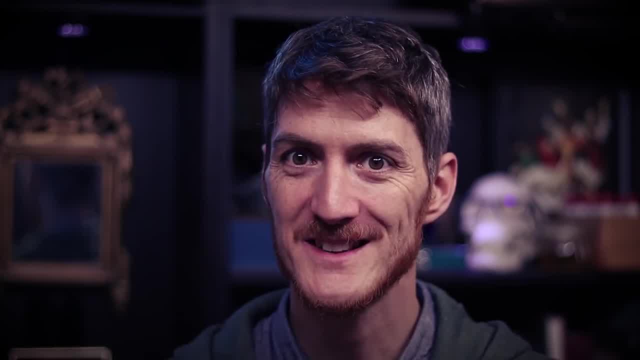 to make the mixing and painting process more fluid and more methodical. With good theory, color mixing is less a guessing game and has a more solid structure. So, hopefully, I hope you enjoyed this video and I'll see you in the next one. Bye, bye. 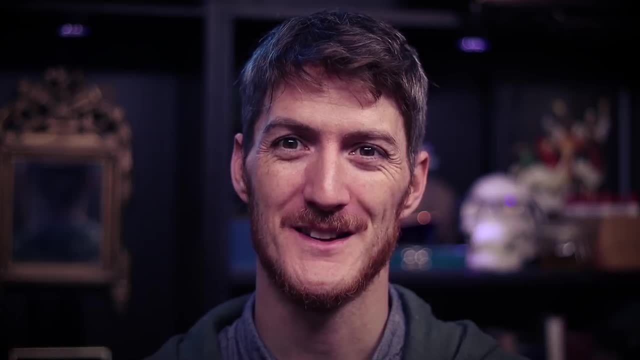 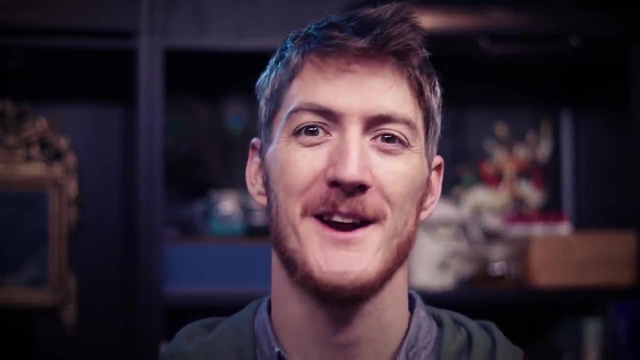 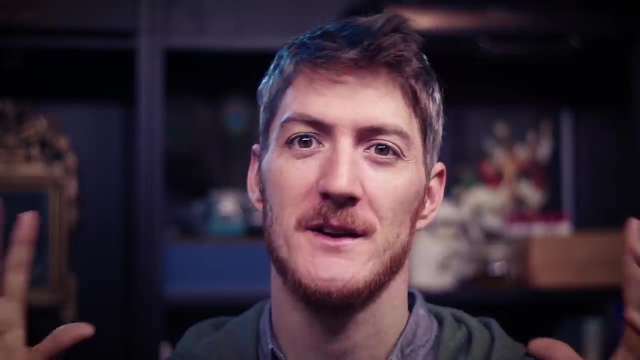 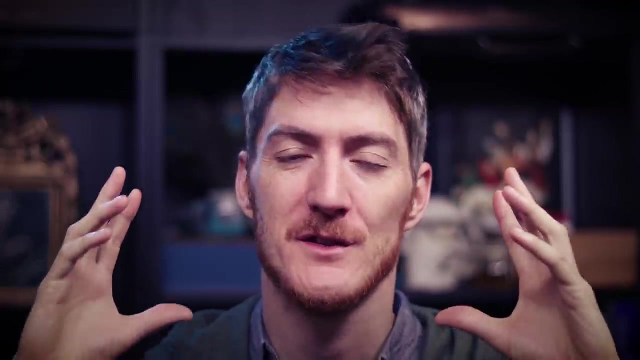 All right, now it's time to talk about the third major role of color theory is composition and harmony. Unfortunately, this subject is so vast that I don't think I'm going to have time to cover everything in this one video, so I'm going to give you just the 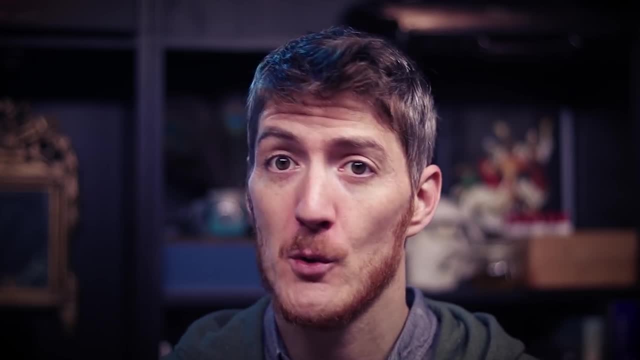 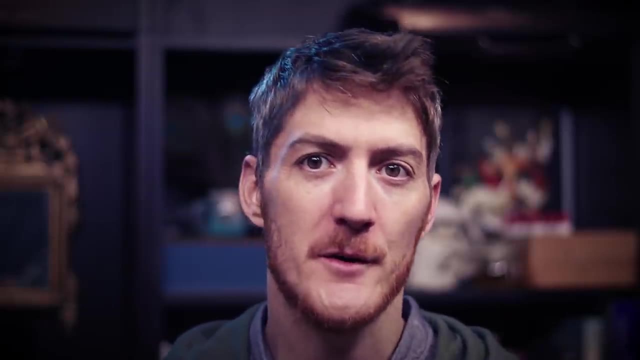 main lines. If you want to learn more, just check out my new course, because I really dive deep into all the possibilities of color composition, color theory and color harmony. So really check out the course if you want to learn more. For this video I'm going to 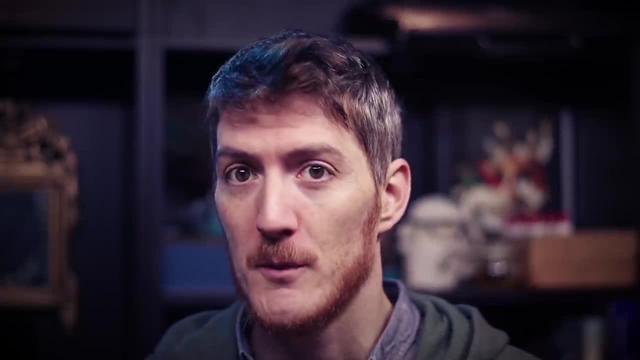 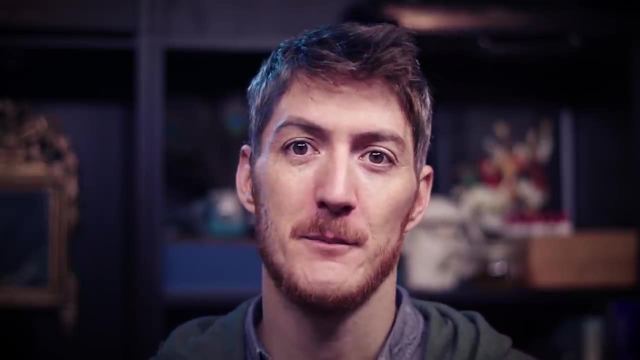 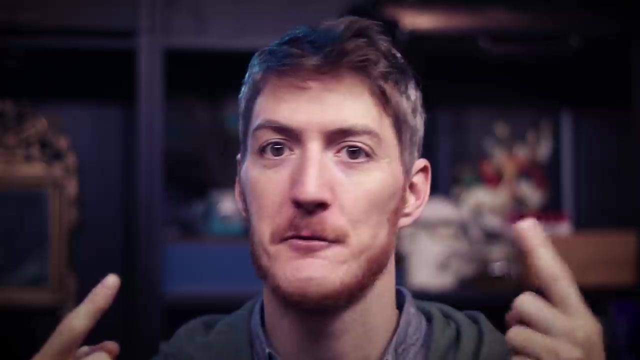 just give you the main lines. Well, and one of the main problems when we talk about color theory and color composition, color harmony especially, is that most of the time people only think about hue harmony, Like: should we put green and red together? because they? 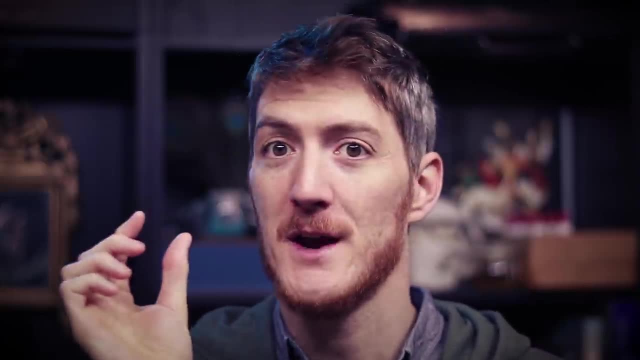 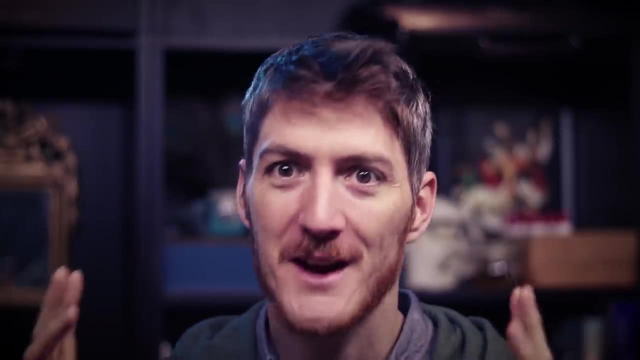 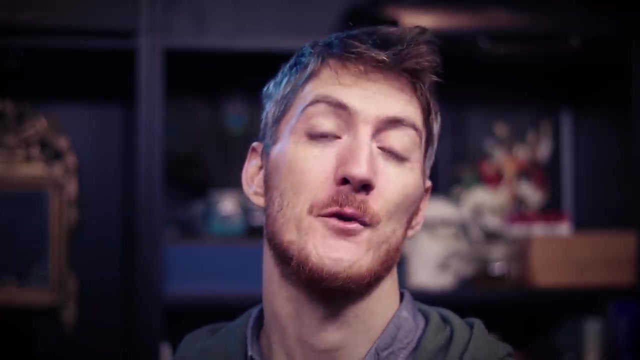 go well together. The problem is that most of the time people are just considering hue, But color isn't just hue. Again, the three dimensions of color, they are here. again, It's a recurring thing, But actually if you really want to explore the full potential of color harmony, 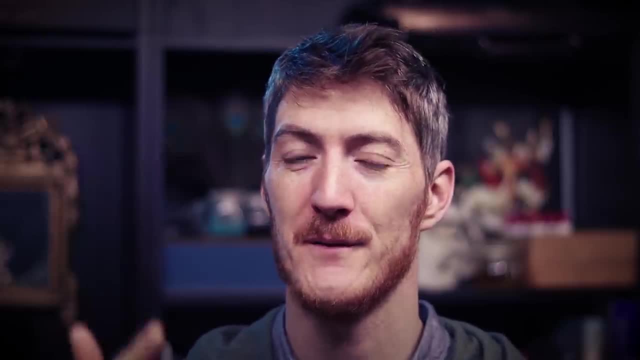 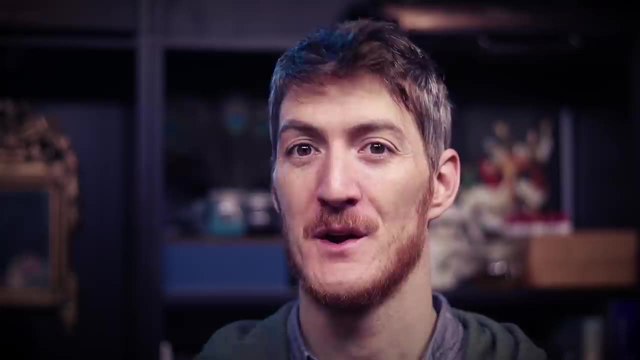 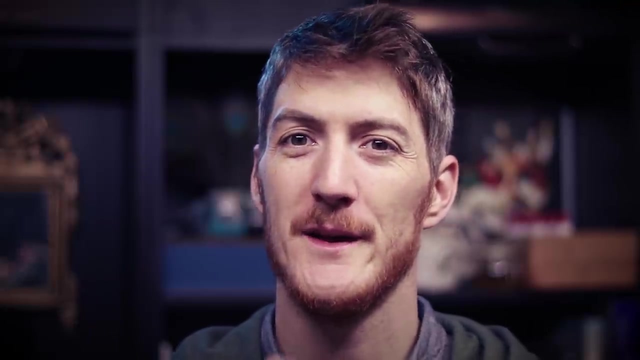 you have to consider hue, value and chroma, And actually hue is probably the least important element to take into consideration when thinking about color harmony, For example. if you compose with value, you'll probably start with a black and white study. 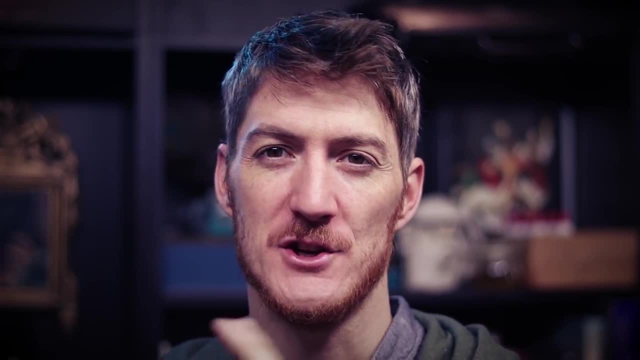 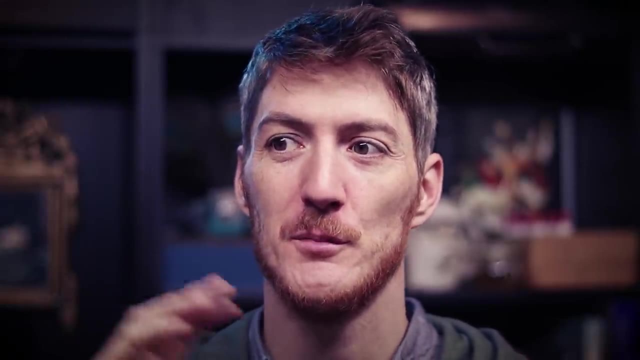 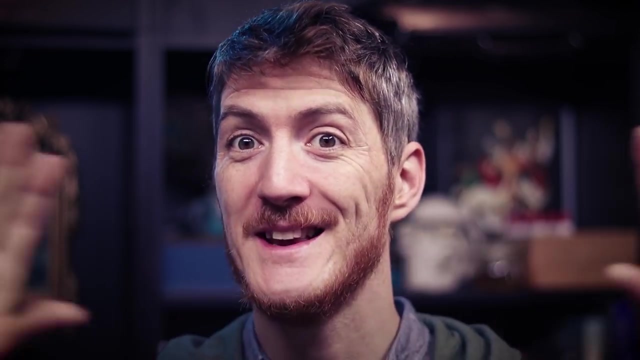 to see how to represent the light and shadows. Should there be a big dark background or should everything be very light? Do you want to put strong shadows? Do you want to put very soft and light shadows? Do you want a very even light? 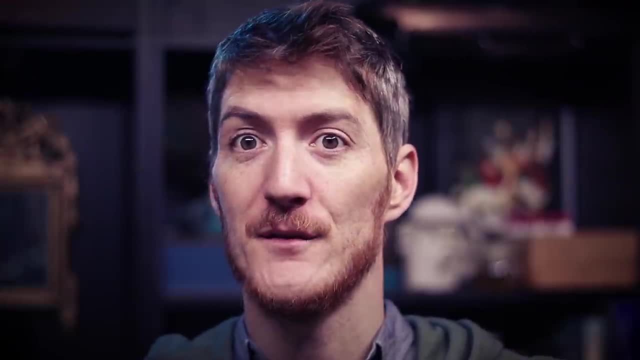 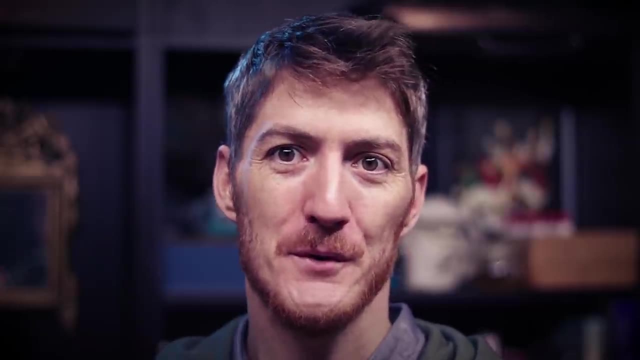 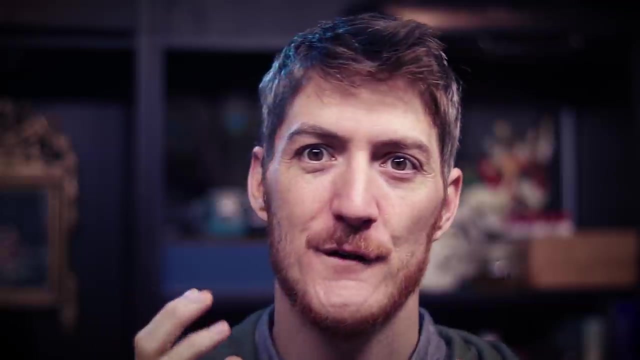 like a big sky making a very diffuse light, or do you want just a simple candle light to light your subject? These things are important. it's not the same to paint this or this. So this is the strength of composing with values. Never forget that. 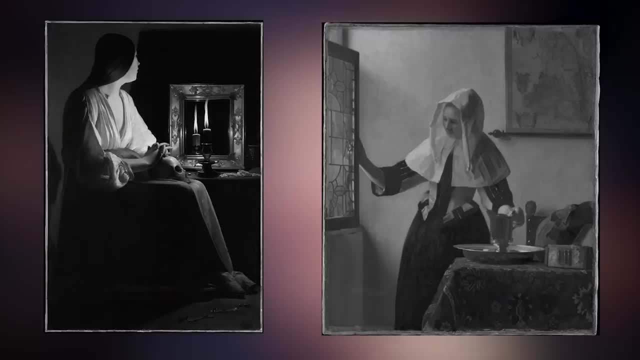 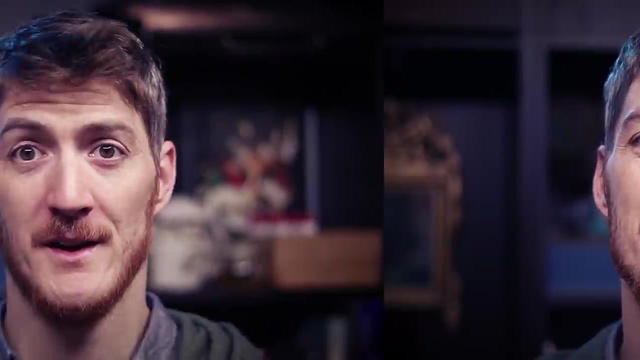 an image should look good in black and white, and if it already looks good in black and white, hue and chroma are just going to be an element that will make it even more rich and more vibrant. Next, we have to talk about composing with chroma. 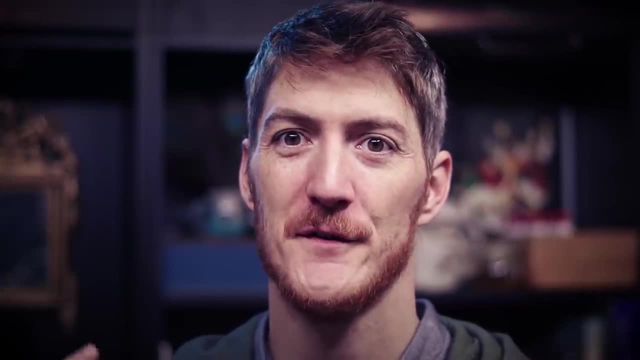 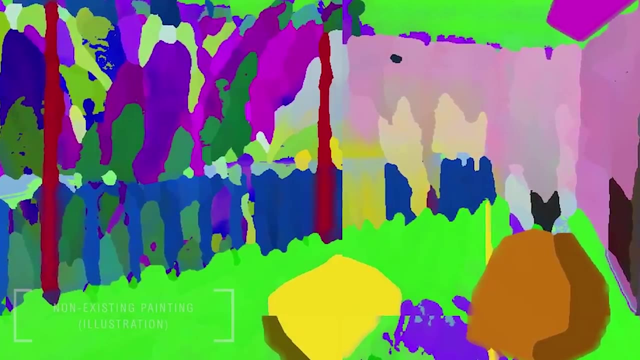 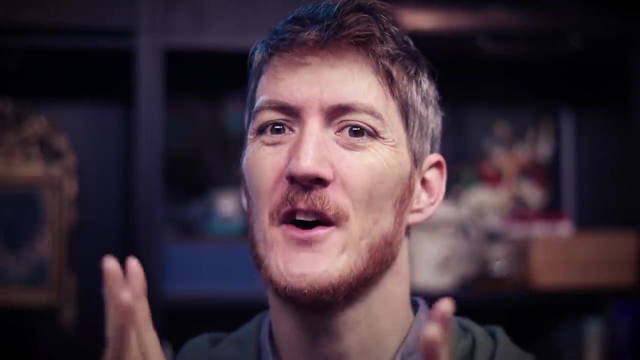 which is also a very, very important part of color harmony. If everything has a super high chroma, well, maybe the picture will be very unappealing, because everything will just scream very loudly and And it's very hard to understand the hierarchy of colors in the composition. 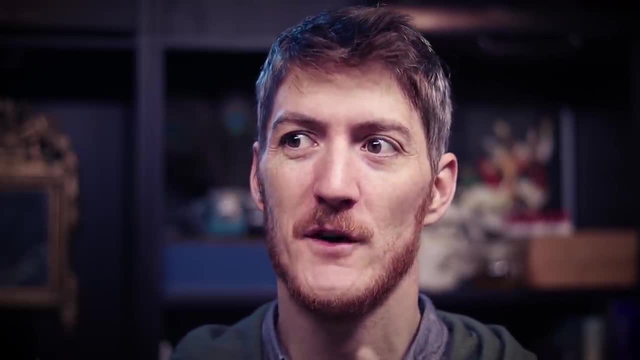 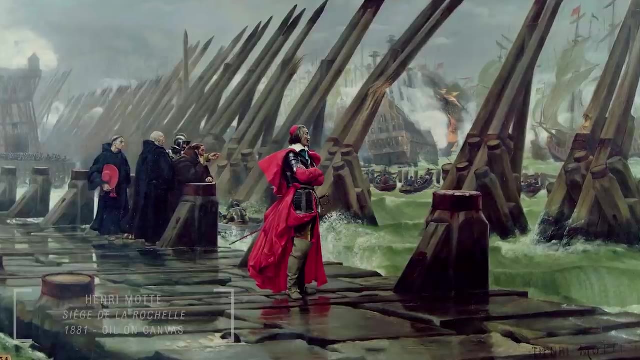 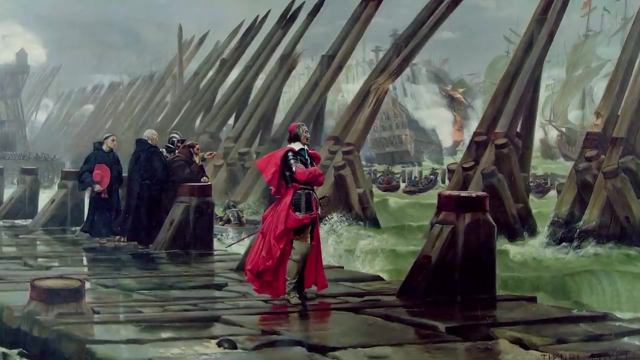 If everything has a super high chroma, it's very hard to understand what to look for exactly, Whereas if everything in the painting is rather dull and just one or two well-chosen colors have a high chroma, then you will focus the eye of the viewers on these specific parts. 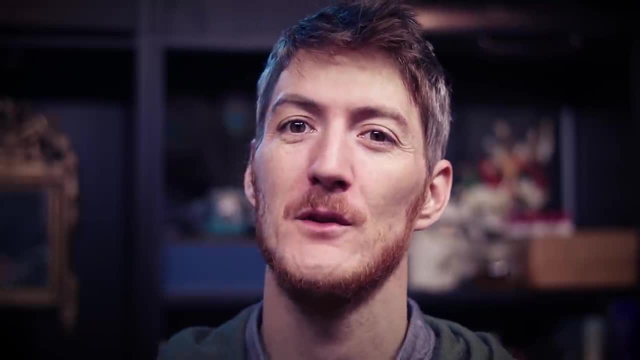 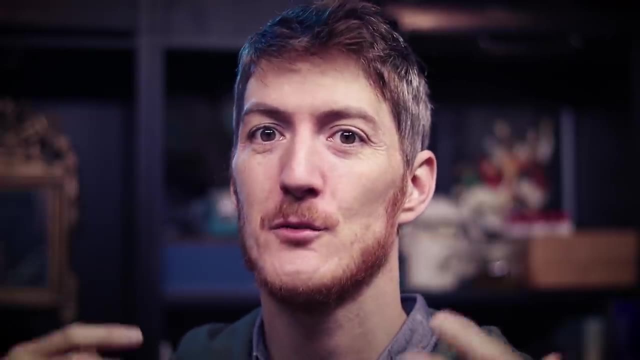 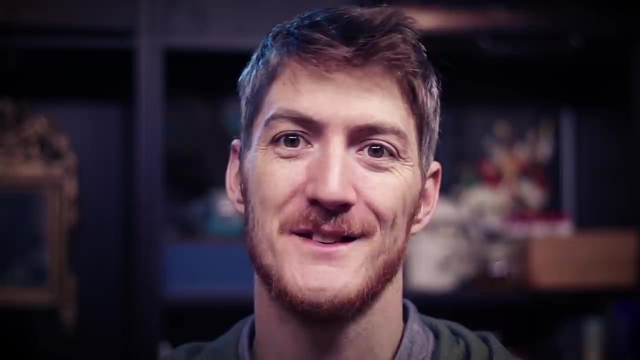 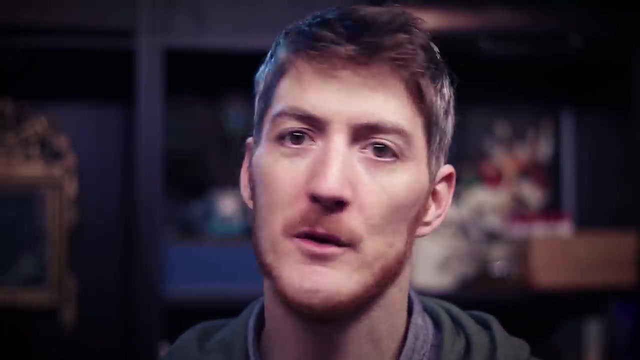 And this will allow you to tell a story. this will allow you to guide the eye of the viewers, And that's actually a great thing, because you can really start using colors to bring a narrative into the paintings that you're trying to create. And finally, composing with hue is the most common thing that most people think about when thinking about color harmony and color composition. 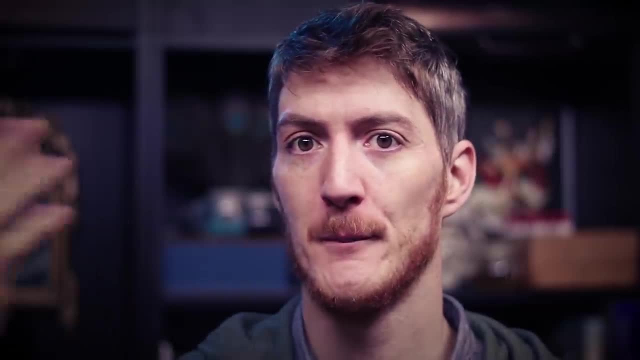 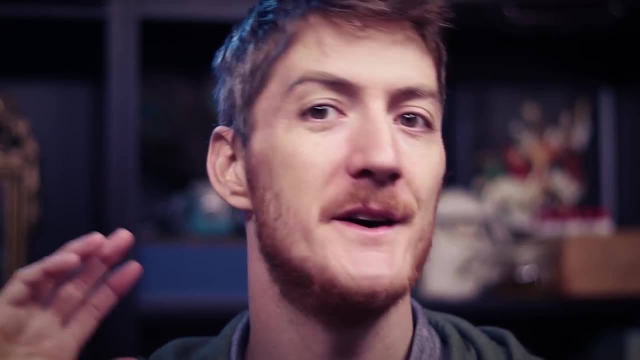 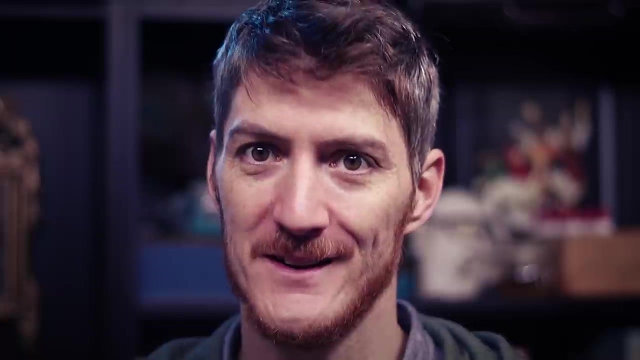 Should you put red and green together? Should you put purple and yellow together? Should you put red, orange and yellow? I mean there are a lot of categories, subcategories, so quite complicated stuff. I talk about it in depth, in my course. I'm not going to dive into it because it would just take way too much time. 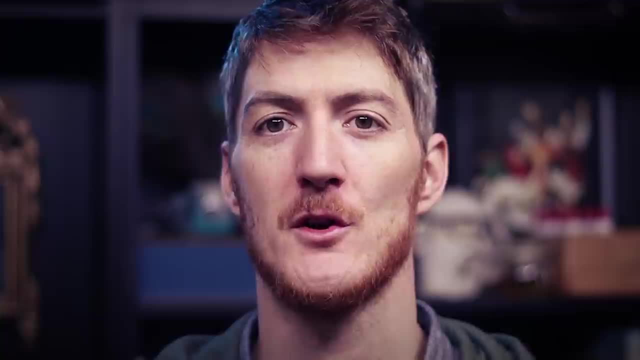 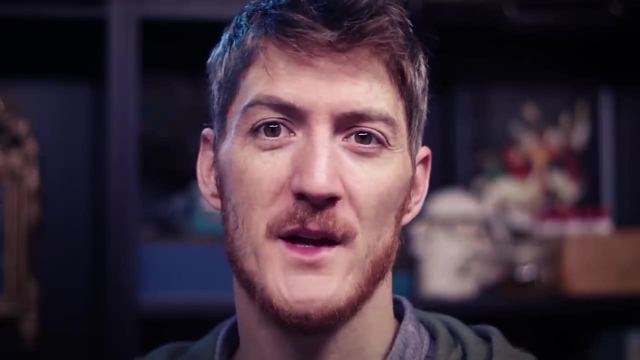 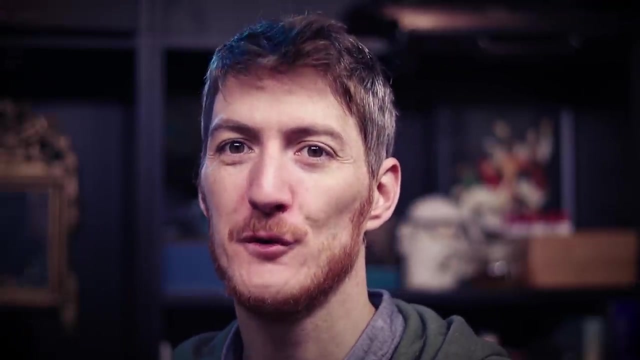 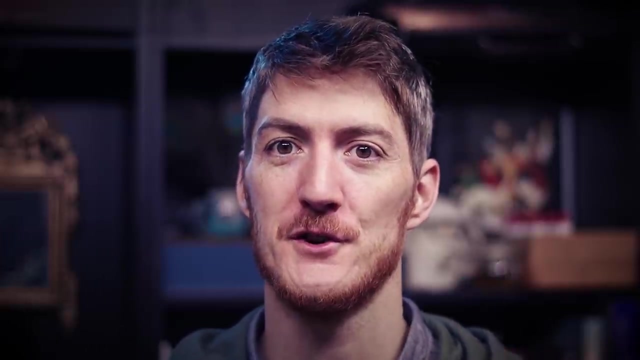 But just know that if you have done a good job composing with values first, if you have done a good job composing with chroma, then composing with hue is just icing on the cake and it's just bringing nice, elegant hues that go well together to finalize an already decently structured composition. 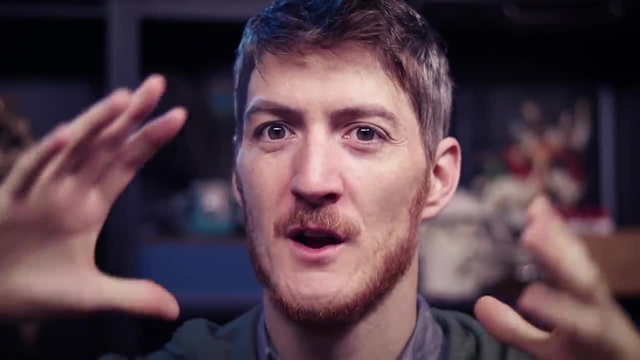 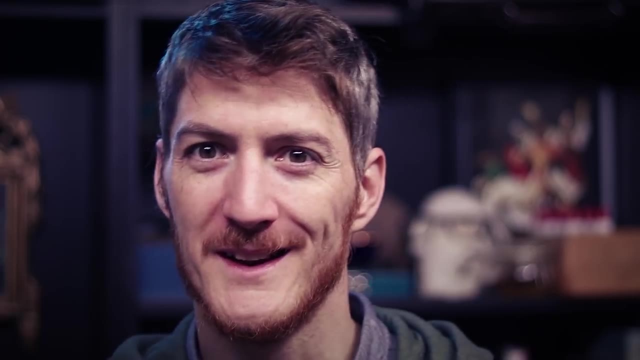 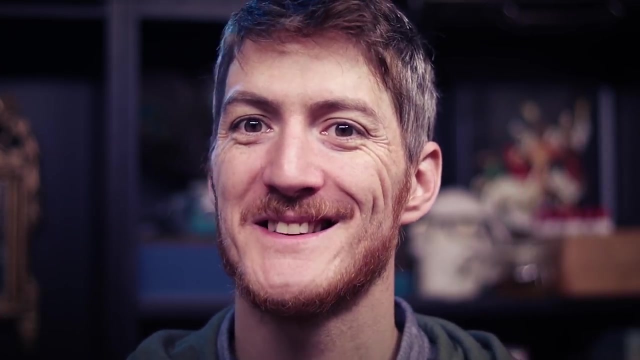 So the value will be the skeleton of the composition, the structure on which everything is based on. Then the chroma is what allows you to guide the eye of the viewer, And then the hue is just what makes, what gives the painting its elegance, its pleasant appearance. 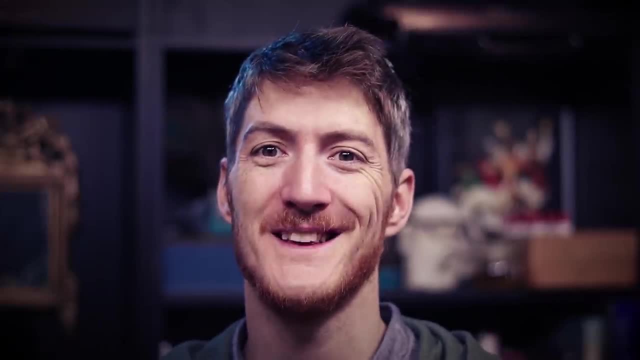 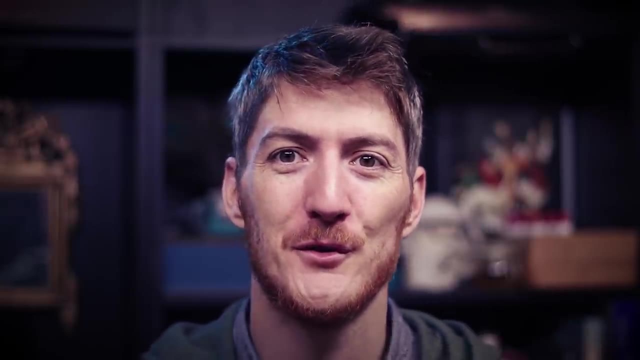 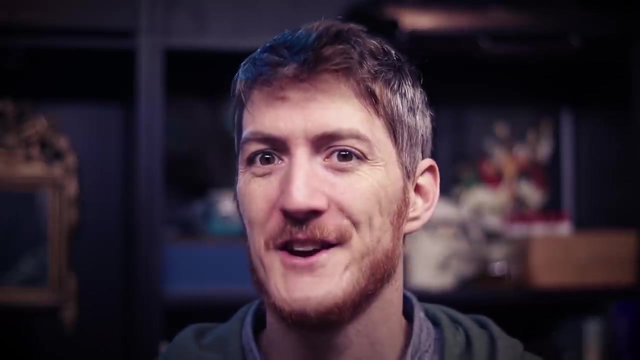 And that's how you compose. The most important is to remember that color harmony, color composition always should have three dimensions. It's very important to explore all the potential of the colors and not just hue. All right, that's it for this explanation.